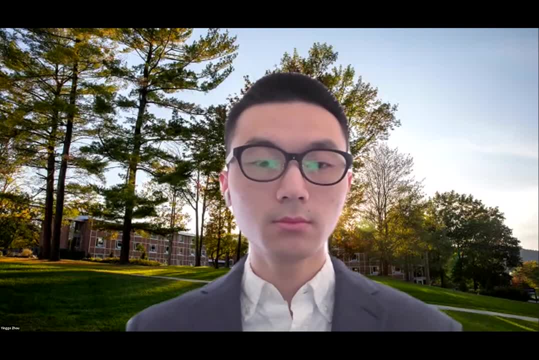 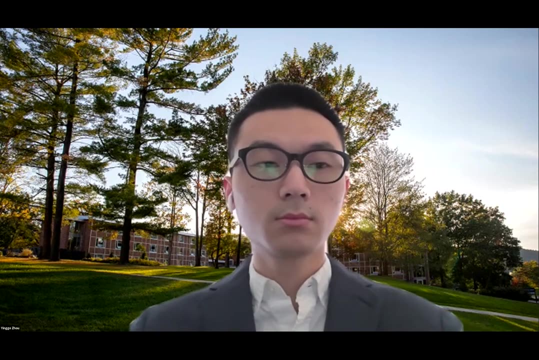 Today's speaker is Dr Yenge Zhao, who received his PhD from the Department of Industrial Manufacturing and Systems Engineering at Texas Tech University in Lubbock, Texas, in 2020.. Dr Zhao earned his bachelor's in mechanical engineering and business administration from Shantan University, China, in 2014, and his master's degree in industrial engineering from Texas Tech in 2016.. 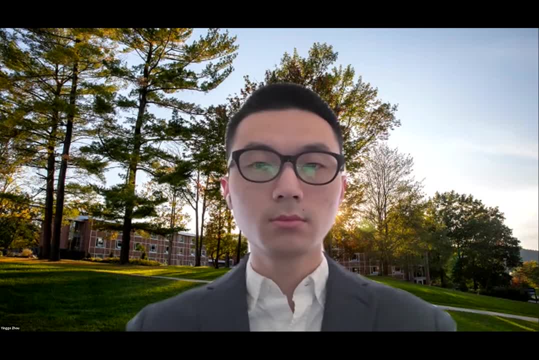 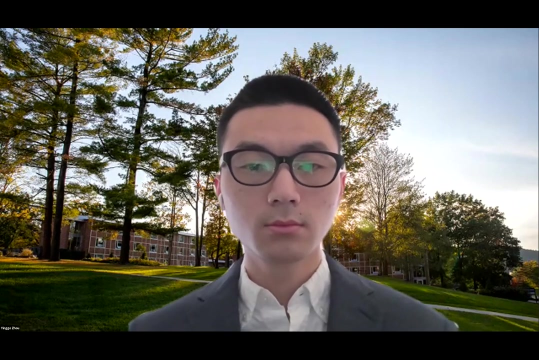 His research focuses on microfabrication and hybrid manufacturing of 3D biomimetic architecture for biomedical applications. He made a major contribution to developing an innovative electrospinning strategy that includes rapid assembly of aligned 3D fiber scaffolds, which create a biomimetic environment to facilitate 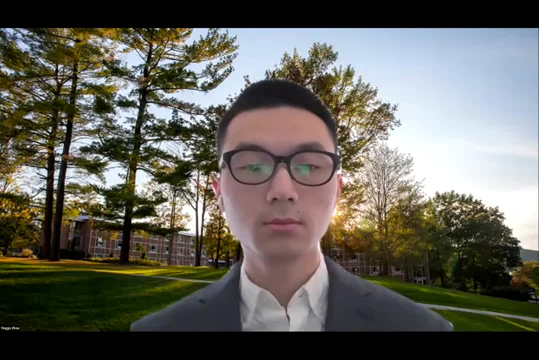 cell morphogenesis. He also conducted pioneering work on the integration of silver nanoparticles and microcurrent of antimicrobial ultrafiltration membranes. His most recent work focuses on rapid fabrication of nanoporous microtubes as artificial capillary vessels for tissue engineering. Dr Zhao has published more than 20 refereed journal papers and conference papers. 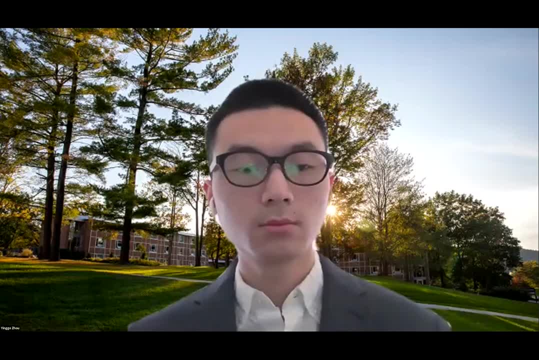 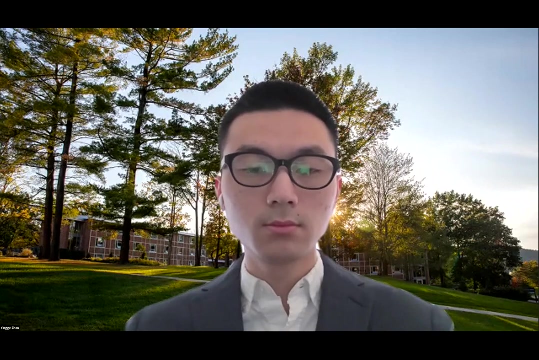 His teaching interests include manufacturing systems, additive manufacturing processes and systems, and biomedical design and manufacturing, and he's also a member of IISC and ASME, So please join me in welcoming Dr Zhao to our webinar series to speak about electrospinning biomimetic scaffolds for tissue engineering. 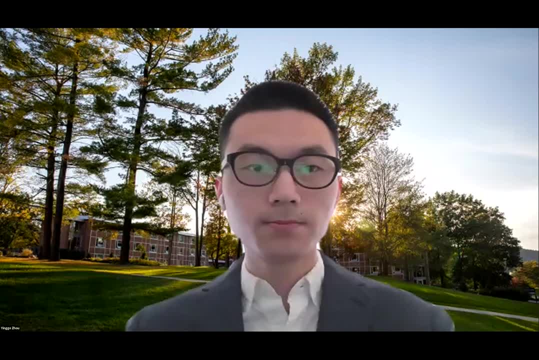 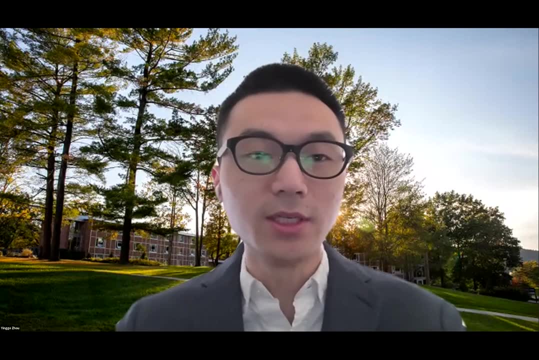 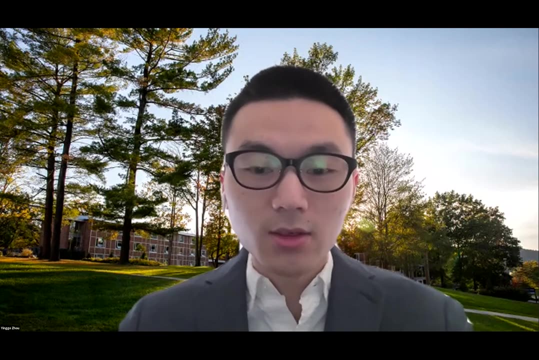 Dr Zhao, thank you again for joining us and I will turn it over to you. Okay, thank you, Professor Cassoni, for your introduction, and good morning everyone in the US and good evening everyone in India and also good afternoon Professor Bruno from Italy. So I'll go ahead and share my screen. 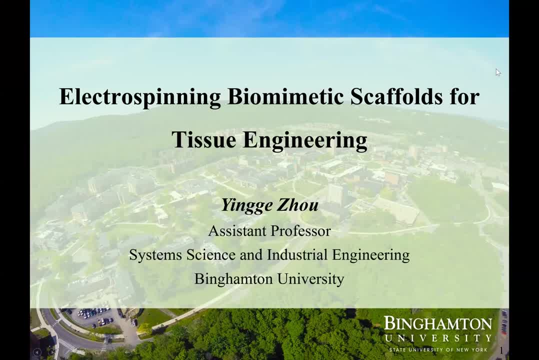 So I'm assuming everyone can see my screen now. Yes, Okay, Okay, perfect. So, as Professor Cassoni mentioned, my name is Inge Zhou. I'm an assistant professor from System Science and Industrial Engineering at Binghamton University. 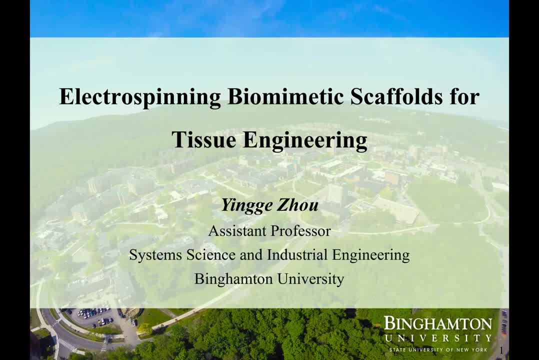 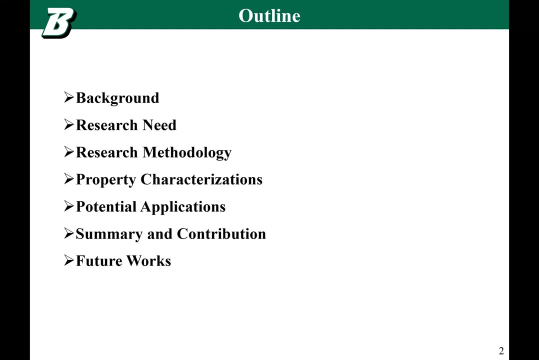 I joined Binghamton University at 2020 and my research focused on tissue engineering, So today's topic will be about electrospinning biomimetic scaffolds for tissue engineering And, without further ado, let's get started. Here is the outline for today's topic. 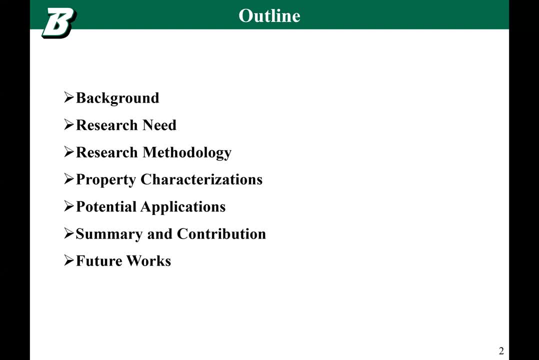 First I'll introduce some of the background in terms of the tissue engineering and electrospinning and then I'll address the research needs as well as research methodology And go through property characterizations as well as potential applications. Finally, I'll go through summary and contribution as well as part of my future works, as I will do in my future career in Binghamton University. 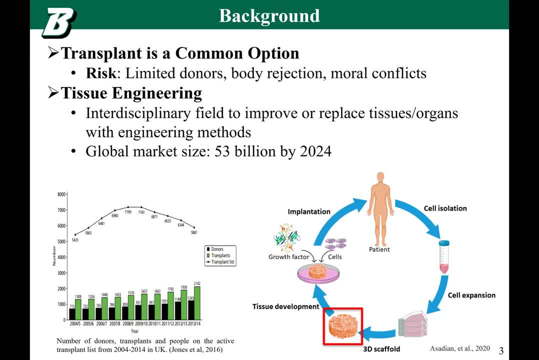 So first we have an organ failure, the first option we think about is always an organ transplant. However, there's always less donor compared to the body who needs donation. So we also face body rejection issue when we are transplanting from someone else, or moral conflicts when we're transplanting from. 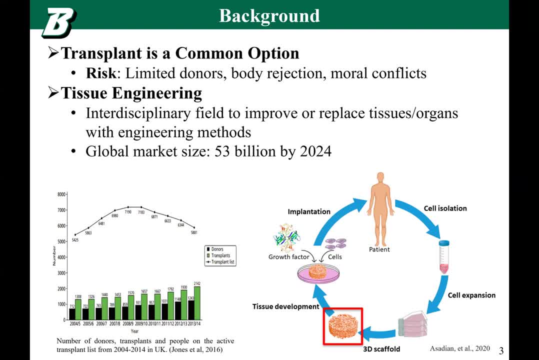 animal models. So in this case, tissue engineering emerged in the last few decades to address those challenges and risks. Tissue engineering is an interdisciplinary field to improve or replace tissues or organs with engineering methods. Its global size is about to reach 53 billion by 2024.. 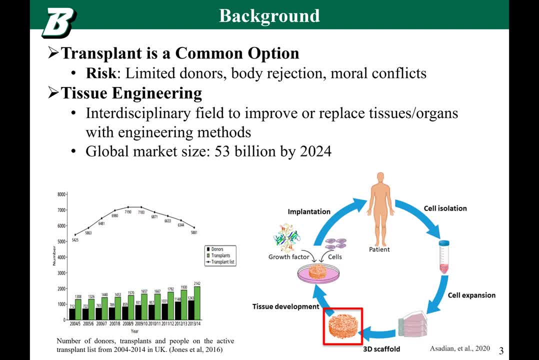 So, in order to repair and improve organ tissues with engineering methods, first we need to isolate the cells from human body and then we also need to expand cells and fabricate some 3D scaffolds to develop a tissue. After we have the cells and scaffolds, the last important factor will be. 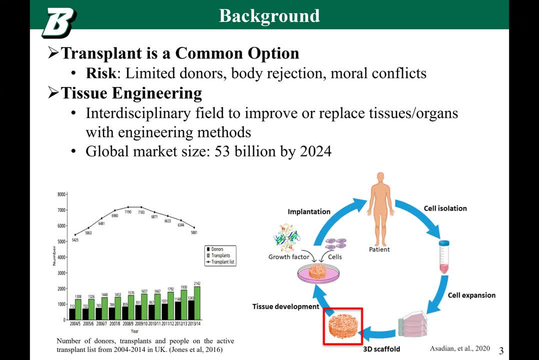 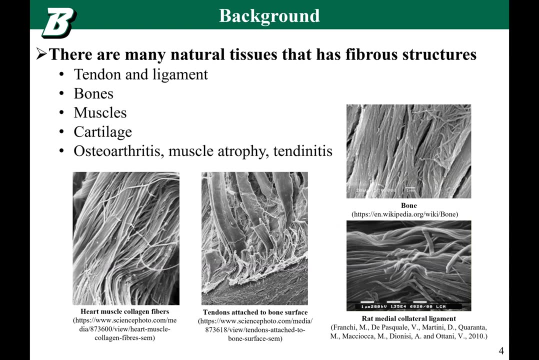 biological factors such as growth factors. So, as industrial engineers, I focus on the fabrication of 3D scaffolds. So, out of all of the tissues in our human body, nanofibers tissues has come to our special attention because there are many natural tissues that have fibers, structures such as tendon. 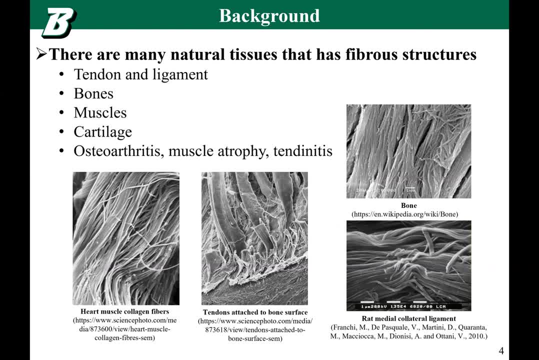 ligaments, bones, muscles and cartilages. Those tissues are related to a major range of disease, such as osteoarthritis, muscle atrophy and tendonitis, as well as cardiovascular disease. So those diseases are infecting more than 50% of populations in the world. 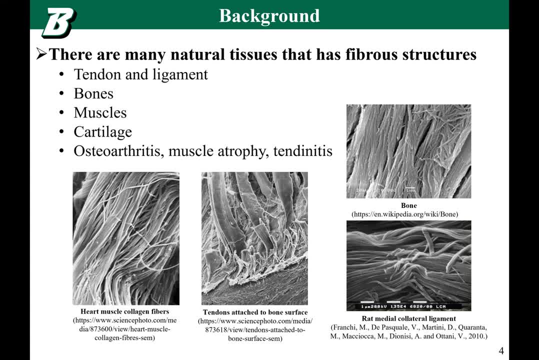 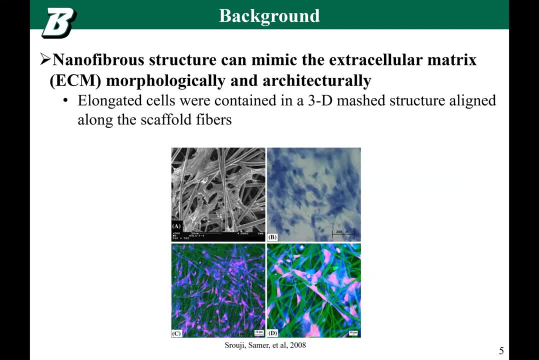 And we need to figure out a way how to mimic these fibers, tissues. So, as we know, nanofiber structure can mimic the extracellular matrix morphologically and architecturally. So in this research we can see that in the artificial, manufactured nanofiber structure, the cells attached on the 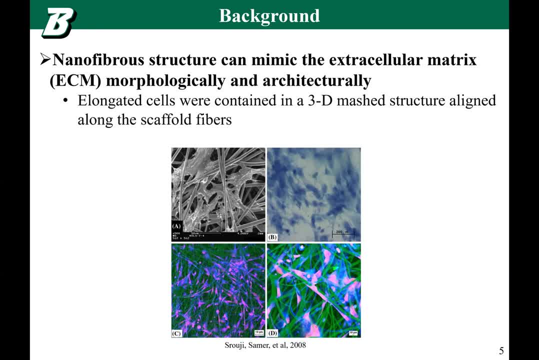 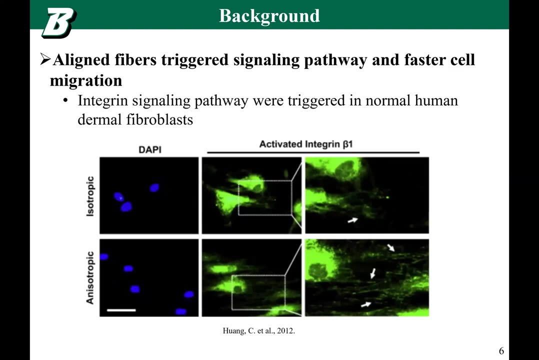 scaffold and were elongated and were contained in a 3D mesh structure. And they were. the cells were growing aligned along the scaffold fibers. We also know that aligned fibers can trigger signaling pathway and faster cell migration. So, based on this research, we see integrating signaling. 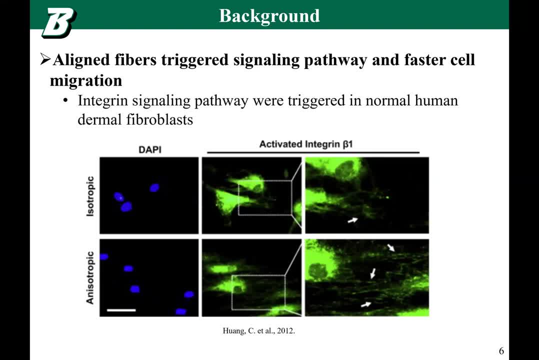 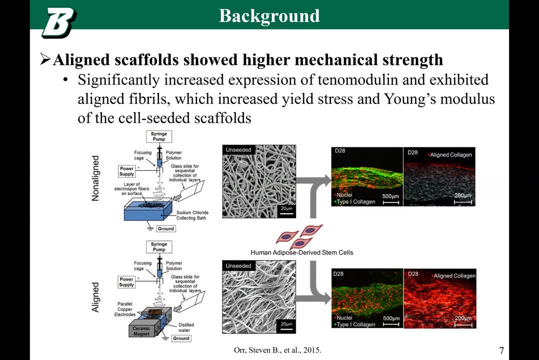 pathway were triggered in normal human dermal fibroblasts when we are fabricating aligned fibers. So aligned fibers can also show higher mechanical strength since they are all aligned in the scaffold. So in this research it shows significantly increased expression of tenomodulin and exhibited aligned fibers which increased eel stress and Young's modulus. 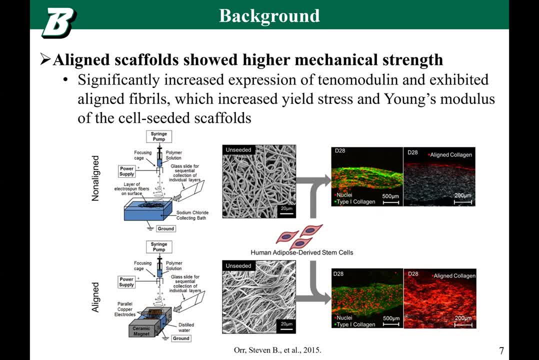 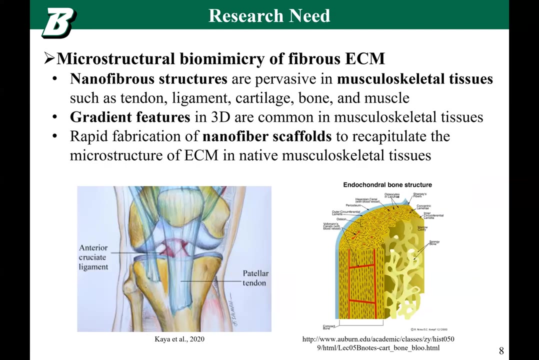 of the cell-seated scaffolds. So, as you can see, not only the mechanical strength of the scaffold can be enhanced, the cell-seated scaffold will also have improved mechanical strength. So now we have the result of the experiment on the cell growth. So the science related to cell growth is most 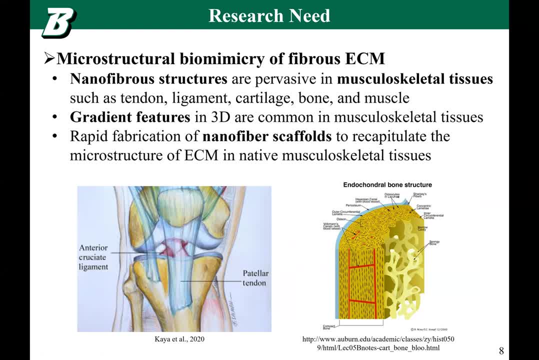 straightforward and the analysis was very effective. The result of the experiment on the cell growth three-dimensional stats and how the cell growth isщееachted is the result of a data analysis. These results have also revealed that aligned fibers can mimic the native fiber's tissues And they are very beneficial for cell growth as well as mechanical strengths. How do we fabricate cell scaffolds that are fiber structures and aligned as well as 3D structures, and can we Bamford that information? We will do this in a moment. 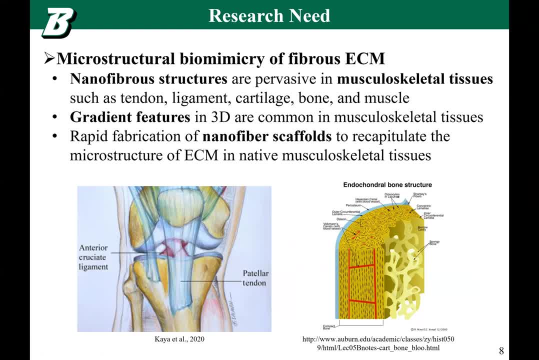 with gradient features. So because here is our search need, because nanofibers structures are persuasive in musculoskeletal tissues such as tendon, ligament, cartilage, bone and muscle, And also there's some gradually changed features in 3D space that are common in musculoskeletal tissues. 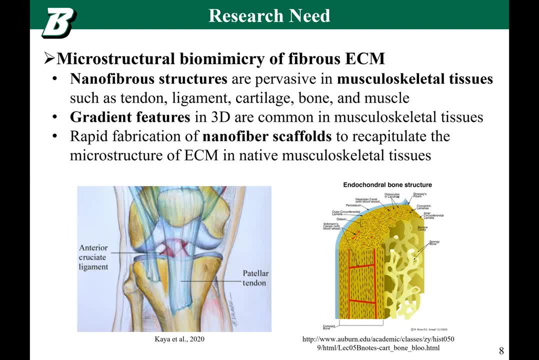 If we take a look at the ligament and tendon, we'll see the fiber density as well as the fiber alignment, as well as the cell alignment will gradually change from one end to the other, because those tendons or ligaments are connecting between bones and between bones to muscles. 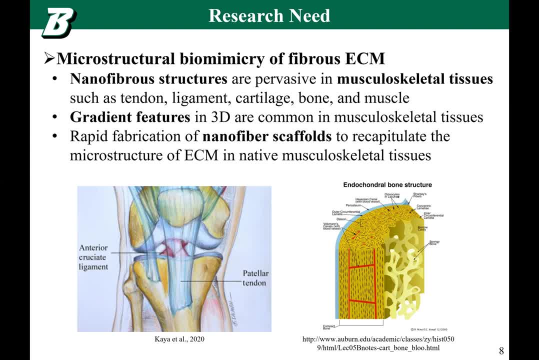 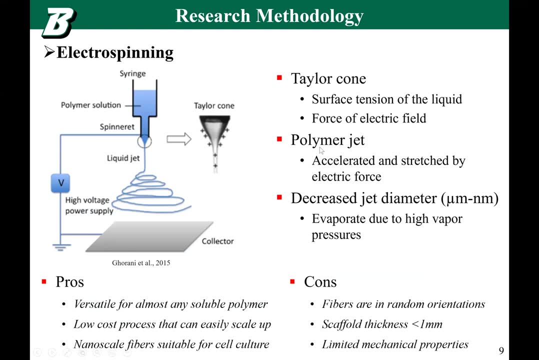 So the rapid fabrication of nanofiber scaffolds- to recapitulate the microstructure of extracellular matrix in native musculoskeletal tissues- becomes our research need. So the research methodology we're introducing here is electrospinning. Electrospinning is a very common way. 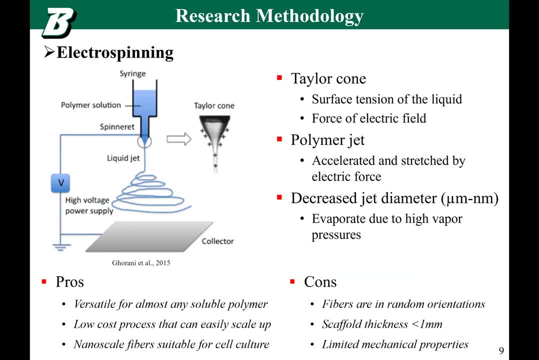 or has been adopted for several decades to fabricate nanofibers and microfibers. So when the high voltage potential applied on the polymeric solution needle tip, the solution will be pulled into a cone shape by electrical force When the electric force exceeds the surface tension. 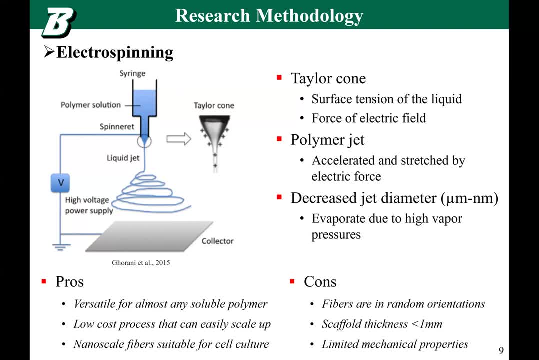 of the liquid. there will be a liquid that will be pulled out from the solution needle tip So as the polymer jet accelerated and stretched by the electrical force, the jet diameter will decrease as the evaporation due to high vapor pressure of the solvent. 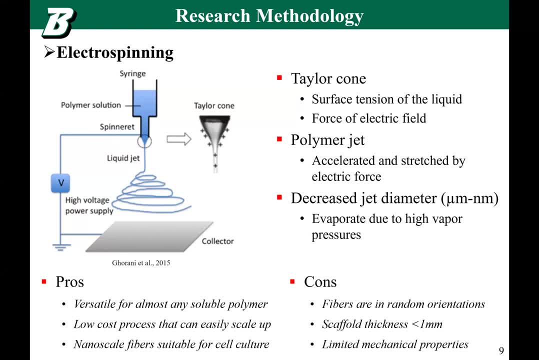 And finally, the jet will become smaller and smaller and we'll get nanofibers and the microsite fibers on our collector. So the advantage of electrospinning is that it's versatile for almost any soluble polymers and it is low cost process that can be easily scale up. 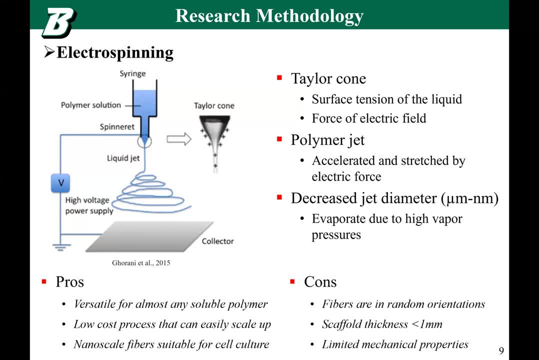 and the nanofibers can suitable for cell culture. So electrospinning can fabricate several tens or hundreds meters of nanofibers in few minutes, So it can be very efficient. However, the fibers are always in random orientation And the scaffold thickness is always smaller. 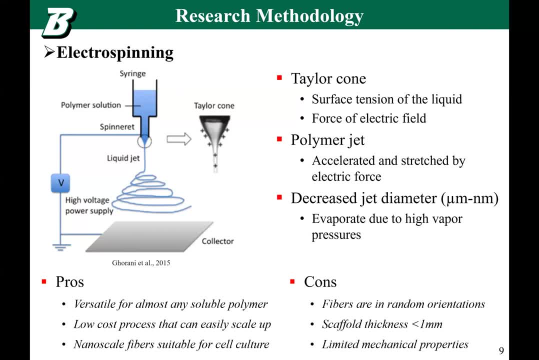 than one millimeters, So, which means they're in 2D scale or in a mat structure, And there's always limited mechanical properties compared to other such as 3D printed or bioprinted scaffolds. So how do we overcome? these are the advantages. 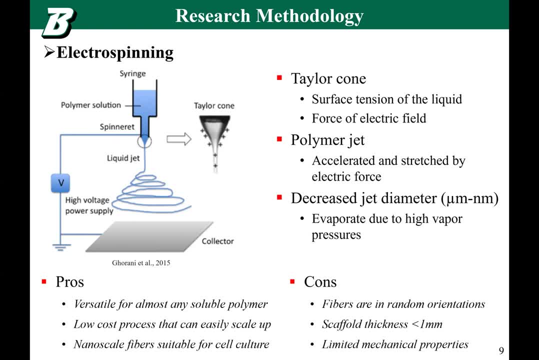 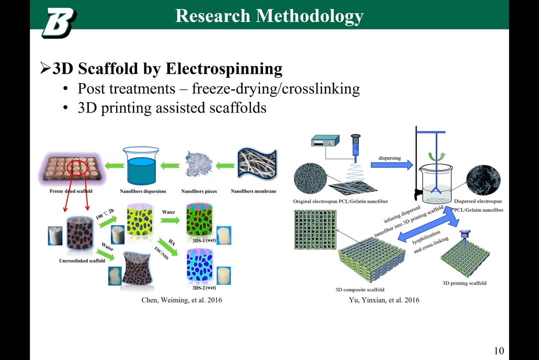 when we are using electrospinning to fabricate nanofiber structures. There's many research endeavors has been done to do that. We have post-treatment such as freeze drying and cross-linking to make the scaffold in three-dimensional and more porous. 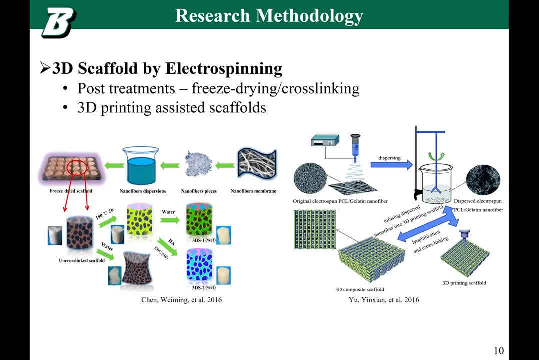 Or we can use 3D printing to print one layer of FDM printed scaffold and another layer of electrospinning fibers to enhance the 3D structure. So this is how we can use electrospinning to fabricate nanofiber structures. 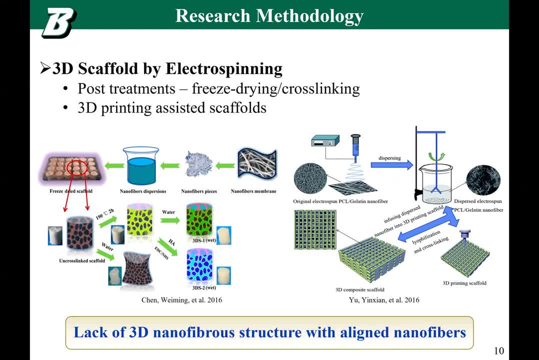 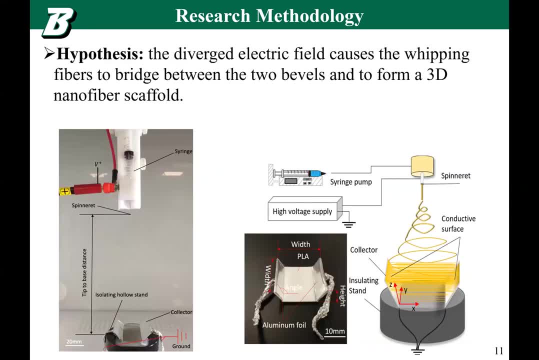 And with the nanofiber structures. However, all of those structures don't have any 3D nanofiber structure with aligned nanofibers, So our strategy is to use a special collector that was specially designed for our research project. So in this collector for electrospinning, 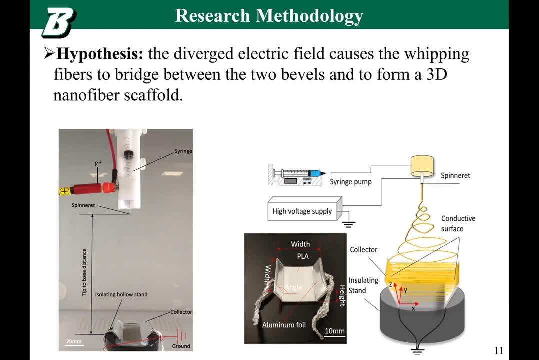 we have two conductive aluminum bevels. These bevels are inclined on the side of the collector And those two bevels are inclined, not horizontal. So we have some inclination angle on the collector And the bottom of the collector is not conductive. 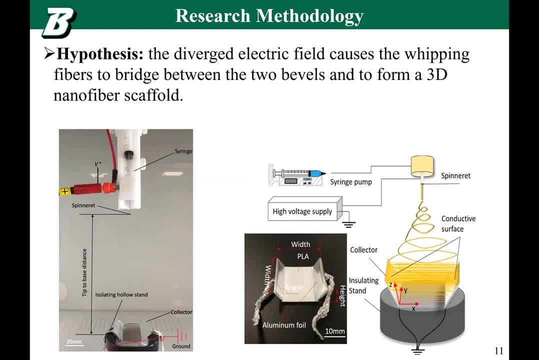 So first we 3D print this shape using a normal FDM 3D printer and then adhere several layers of aluminum foils into the bevels, onto the bevels, And then we put the bevels into the bevels. 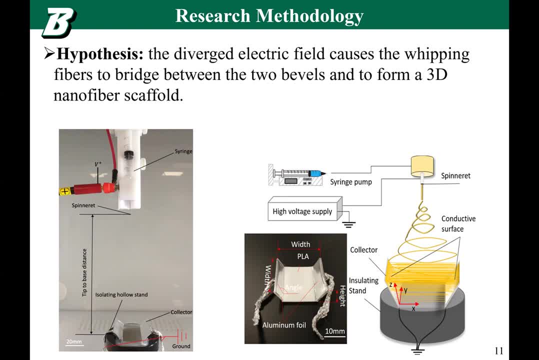 And then we'll place this special collector on our platform beneath the electrospinning spinneret. So the spinneret will be placed on the center above of the collector And the fibers will bridge between the two bevels from bottom to top in a additive manner. 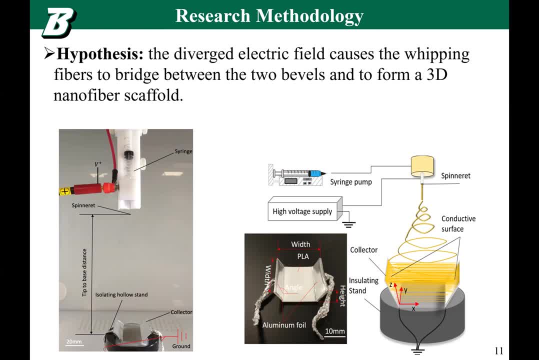 So our hypothesis is that the diverged actual field will cause the whipping fiber to be removed from the bevels. So our hypothesis is that the diverged actual field will cause the whipping fiber to be removed from the bevels. So our hypothesis is that the diverged actual field will cause the whipping fiber to be removed from the bevels. 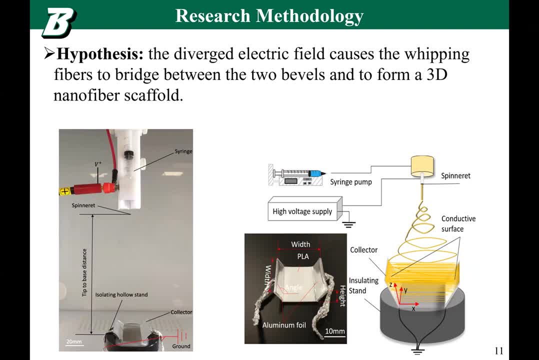 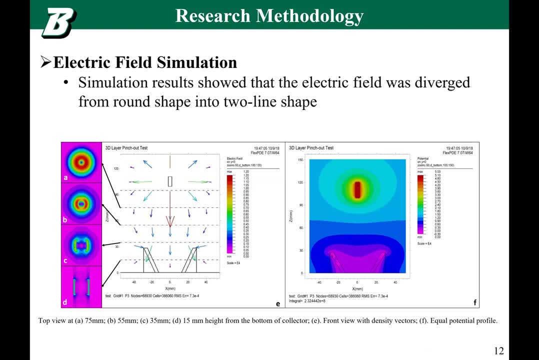 So we have two many different videos to bridge between the two bevels, to form a 3D nanofibers And in order to value the hypothesis, a simulation of the electrical field has been down has been down using flax PDE software. 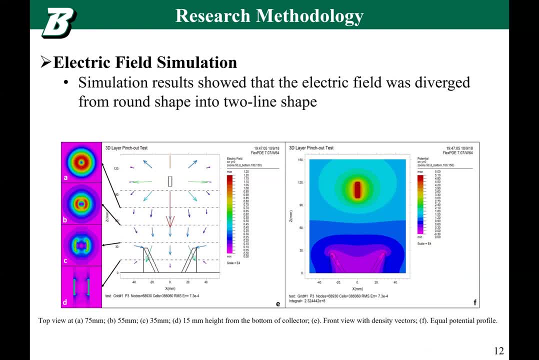 So, as you can see, the electrical field gradually changed from a round shape to a two bevels shape, gradually changed from a round shape to a two bevels shape. This validate our hypothesis that the bits, that is, the white ball for the bevels- 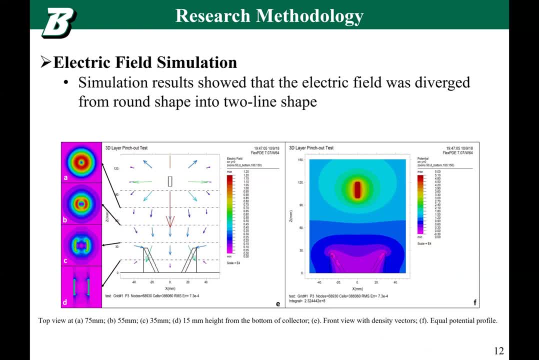 becomes opaque because they are that very, very cloudy. Because if you were to take two DVD here but�� put it in the much, much lower orientation, you would. we're not able to handling work like that. the electrode field has been diverged to a two bevel shape. 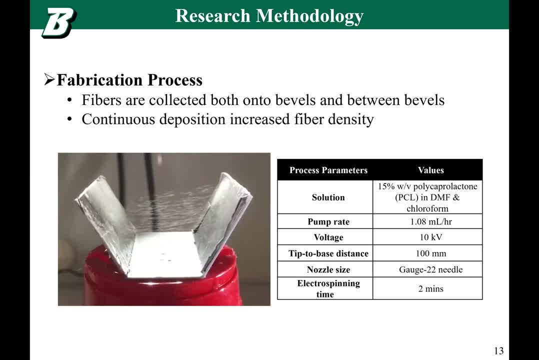 And after the validation of our hypothesis, we select PCL in DMF and chloroform solution, 15 percent weight to volume ratio, and we optimize the pump rate, voltage and tip to base distance, as well as electrospinning time to fabricate the scaffold, As you can see in the video, the fibers: 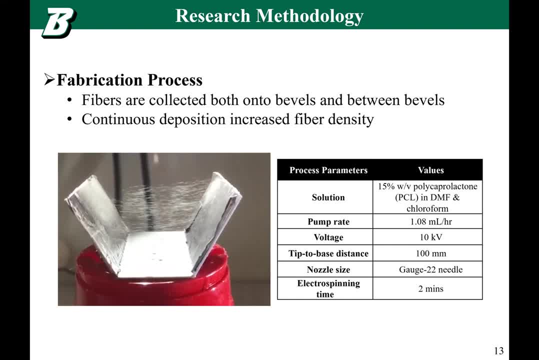 are bridging between the two bevels and are forming a 3D-aligned nanofibers scaffold, And the fibers are collected both onto the bevels and between the bevels, and continuous deposition increases fiber density. Now that we have the scaffold, we want to know. 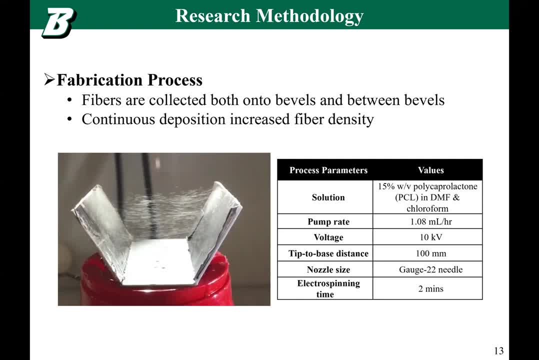 what kind of heat is being produced in the scaffold. So we select PCL in DMF and chloroform solution and we optimize the pump rate to volume ratio effect can affect the fiber diameter or fiber density, as well as fiber alignment. 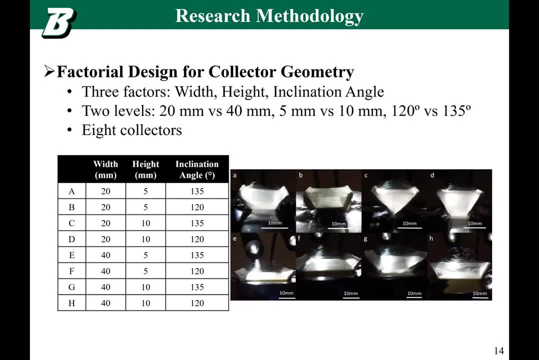 So, in order to investigate the effect of collector geometries on the fiber diameter, fiber density as well as fiber alignment, we designed a factorial experiment that includes two levels for collector width, two levels for collector height, as well as two levels for collector inclination angle. So totally, we got eight different collectors and we fabricate. 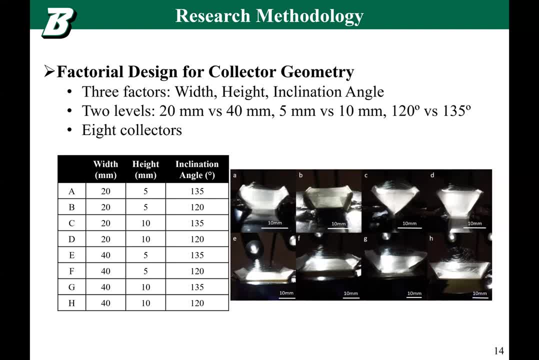 eight different scaffolds. So now that there's eight different scaffolds, it is very hard for us to use the microscope to characterize the fibers, since they are in three different levels. So we need to figure out a way to convert the fibers in 3D scale into 2D scale. So the measures 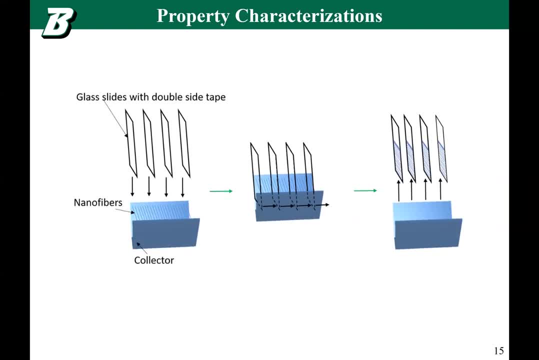 we're adopting here is to use different glass slides with double-sided tape to insert from top to the inside of the scaffold and then to the outside of the scaffold. So this is a very simple way to convert the fibers into 2D scale. So the next step is to use the microscope to 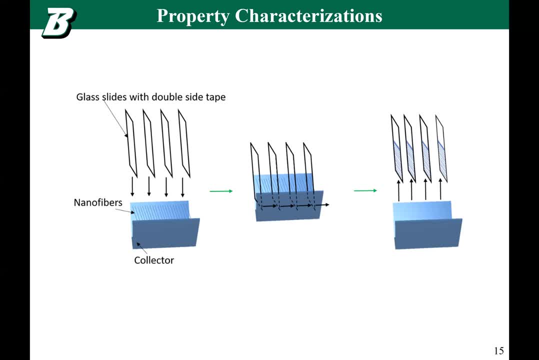 swipe horizontally to collect the fibers in different sections. So, for example, for this one collector we used four glass slides to section the scaffold into four different sections, And after we horizontally swiped the collector, we'll obtain four glass slides with different nanofibers from bottom to top, And then we'll measure the. 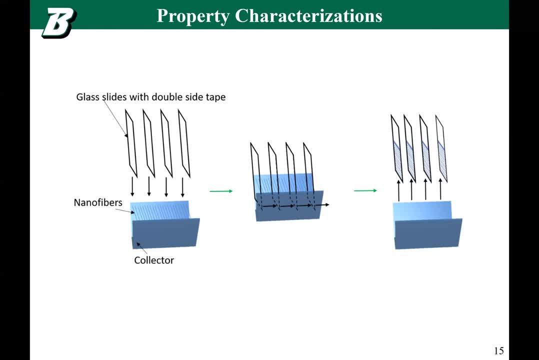 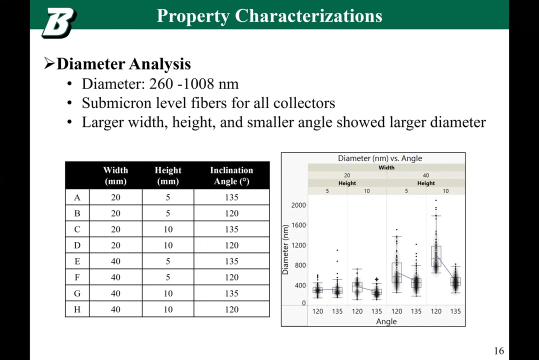 fibers on each glass slide from the bottom to top and separate the glass slide by one millimeter distance. This means for every one millimeter we'll take a microscope or SEM image to characterize the fibers And after fiber diameter analyze in a microscope. we'll see that the fiber diameter 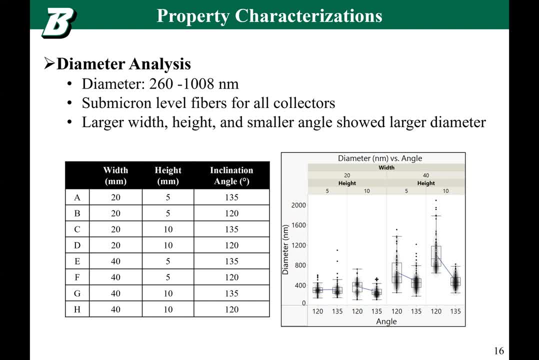 averagely range from 260 to 150 mm And the fiber diameter average range from 260 to 150 mm. 1000 nanometers. This means all fibers are sub-micron level or nanofiber level- nanoscale. 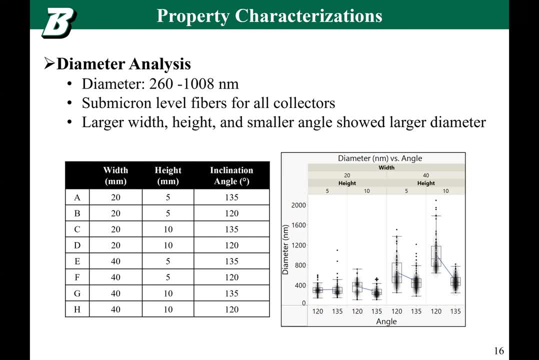 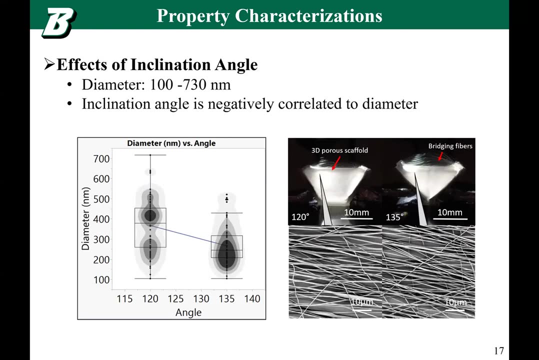 level And we can see for fiber diameter. if we increase the collector width and height or decrease the collector inclination angle, we'll always get bigger fibers. And if we take two scaffolds with different inclination angle, out from the eight different collectors, we'll see. 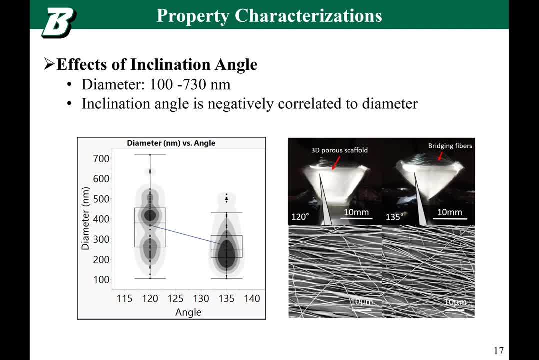 that the fiber with lower inclination angle will have a significantly higher fiber diameter, And you can also see from the SEM image that the fiber orientation are highly aligned, which means we successfully fabricated aligned scaffolds, And for these two collectors the diameter ranged from 100 nanometers to 730 nanometers. 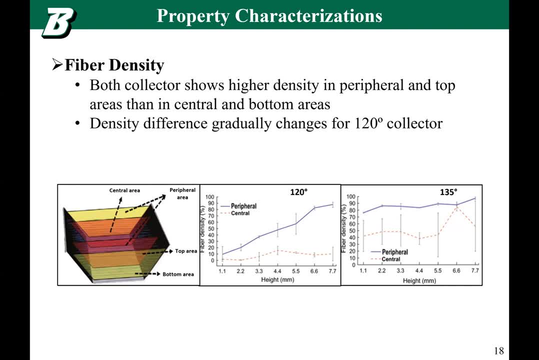 So what about the gradually changed features that we just mentioned to mimic the native tissue, such as tendon ligament, that has gradually changed features from one end to the other? Well, so we separate our scaffold into peripheral error and central error And we compare if there's any fiber density and fiber alignment difference between the peripheral 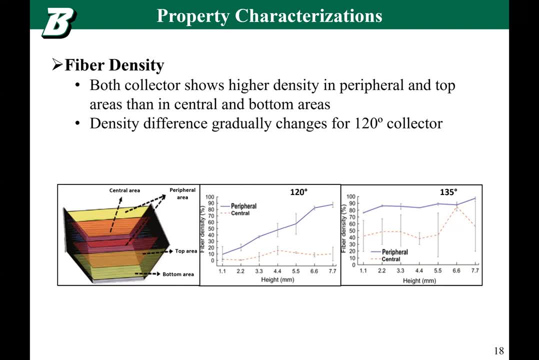 error and central error. So when we take a look at these two different collectors with different inclination angle, we can see that the fiber density for central error is always lower compared to the fiber density for peripheral error. This means we have more scaffold on the peripheral of 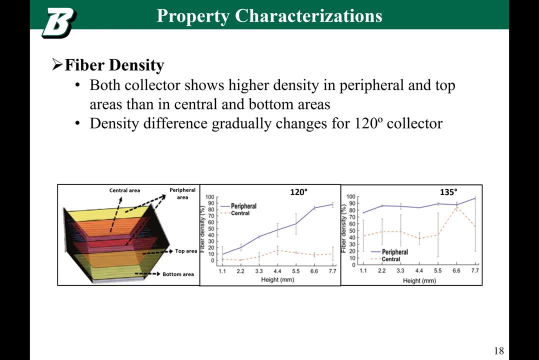 the collector compared to the inside of the collector, And we also noticed as the height of the selector increased from 1 millimeter, 1.1 millimeter all the way to 7.7 millimeter. The difference between the peripheral error and central error also increased. 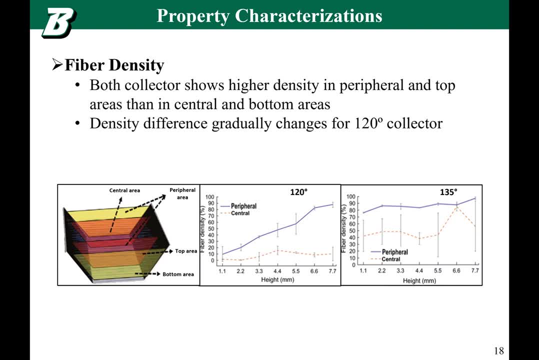 This means, when we are looking from bottom to top, the fiber density are gradually changed compared to peripheral error and central error. However, for the 135 degree collector, the gradually changed pattern is not that obvious. So this means that the collector inclination angle 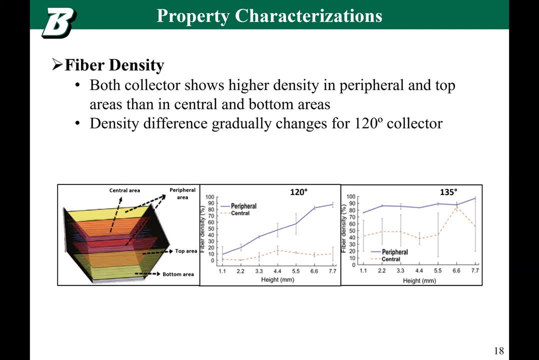 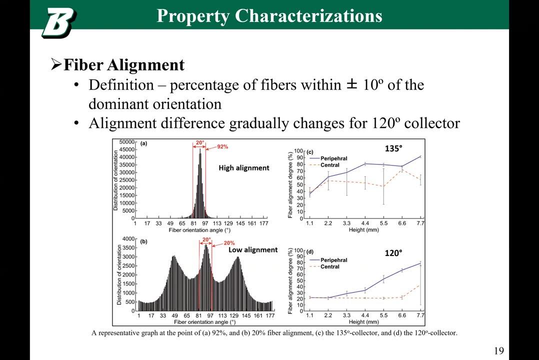 can change the gradient pattern compared to peripheral error and central error in terms of the fiber density. So what about the fiber alignment? So it is: first we need to define how to measure the fiber alignment. So, for example, we have four different glass slides for one collector and we took one SEM or microscope image at 1.1 millimeters. 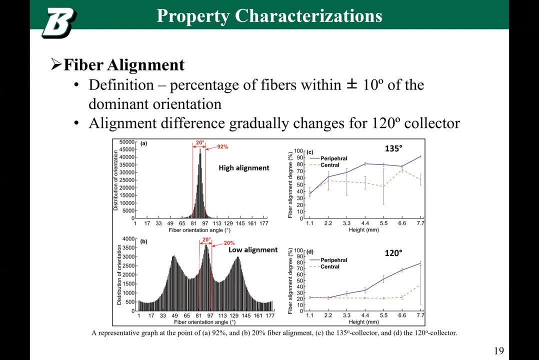 height difference. So after we have so many SEM or microscope images for each image, we'll use the image j to analyze if there's a dominant fiber or a non-dominant fiber alignment. So this is the dominant fiber orientation And if there is a dominant fiber, 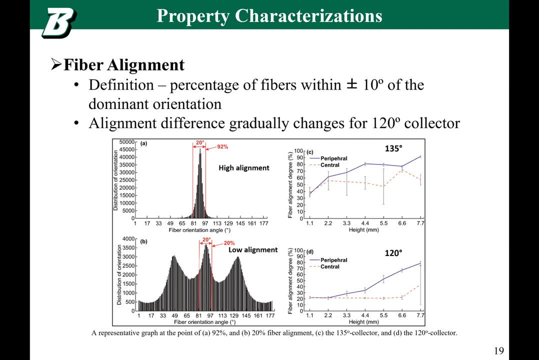 orientation, how many percentage of the fibers are within plus or minus 10 degree of the dominant orientation. That's the 20 degree range, For example, for point A, which we do have, point A here for um 135 degree collector. 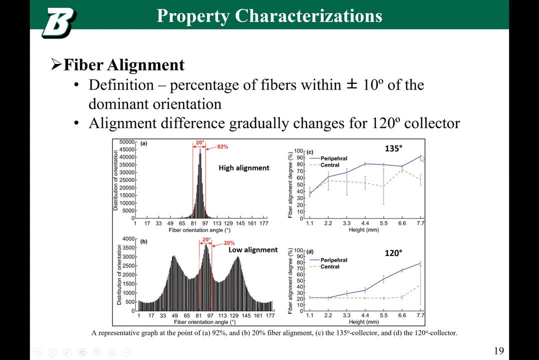 and peripheral error and at 7.7 millimeter height. For this point, we took a SEM image and we found out that 92% of the fibers are within plus and minus 10 degree of the dominant orientation. So we say this point: 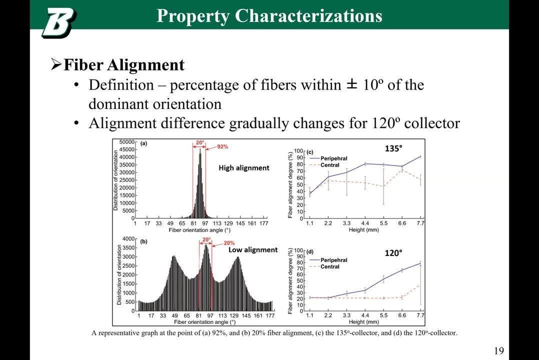 or this area is highly aligned And for this point B we only have 20% of the fibers are within plus or minus the dominant ten degree of the dominant orientation. We say this point or area is lowly aligned. So after we have alignment data for every point or area, we can plot the 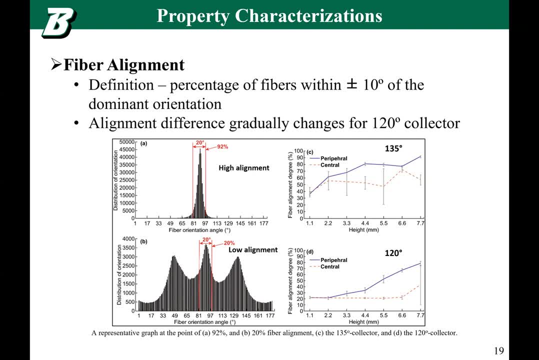 alignment gradient features for every collector. So again, let's take a look at these two different collectors with two different angles. We can see for 120 degree collection. again, the channeled Nation is well connected. so, as you see in the repositiveMPM results, i'm looking. 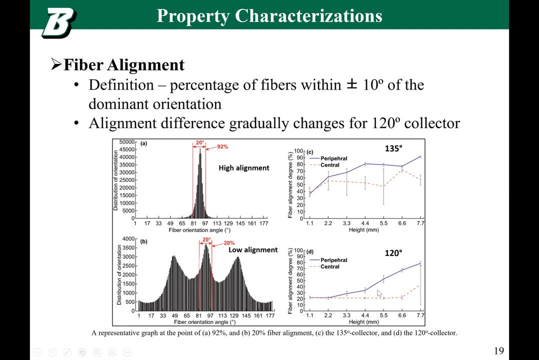 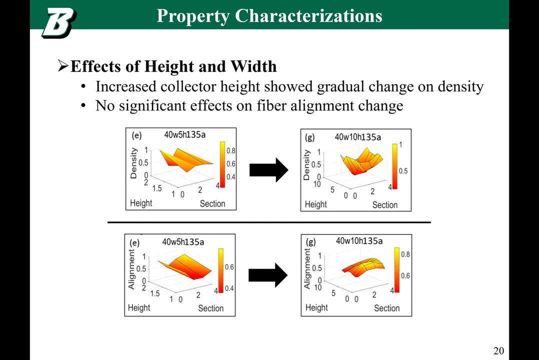 central area has lower alignment level overall. However, the distance between the difference between peripheral area and central area gradually increased. when we're looking from bottom to top, This means the inclination angle can also change the alignment level from bottom to top of the scaffold. So we also did a MATLAB plot to plot every fiber density and alignment. 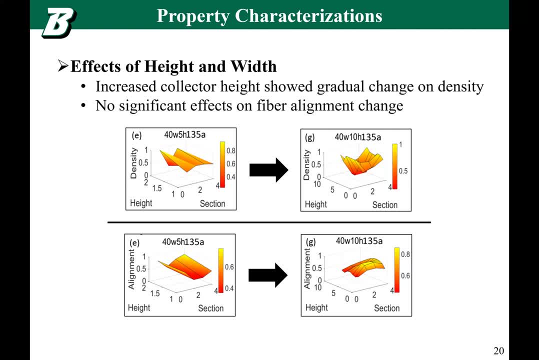 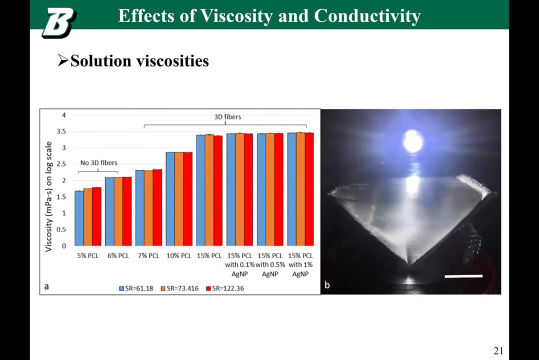 point see if there's a significant change when we are changing the collector height and width. And we found out that there is. an increased collector height showed gradually change on fiber density but there's no significant effect on fiber alignment change. So after we investigate the effect of collector geometry, we found out that the preferral 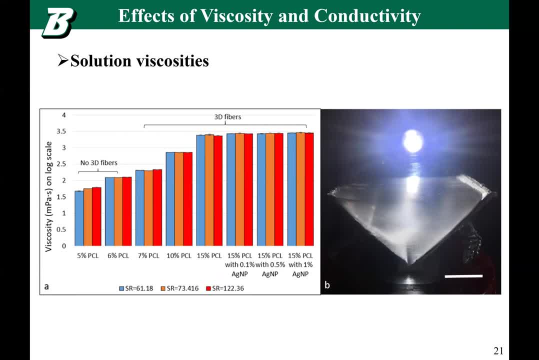 error always have more fibers compared to the central error. So this means the central error of the scaffold may not have efficient fibers for stealth to growth. So we are wondering: if we increase the solution viscosity or solution conductivity, can we overcome the electrostatic impulse, repulse force between the deposit central fibers and 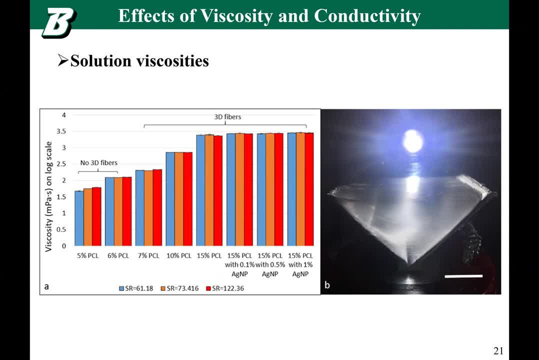 the preferral fibers so that we can deposit more fibers in the central error and get a more homogeneous scaffold overall. But we still want the gradient features, of course. So and also we're just curious: if we decrease the solution viscosity, will we still get? 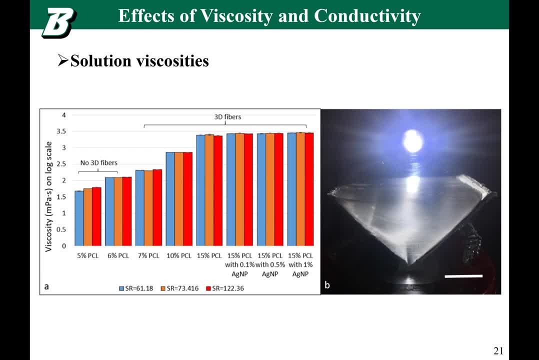 fibers in 3D space. So here is why we designed another experiment, that with different levels of the solution viscosity, as well as different levels with solution conductivity. So how can we increase the solution conductivity? We incorporate different percentage Of the silver nanoparticles into our solution to increase the solution conductivity. 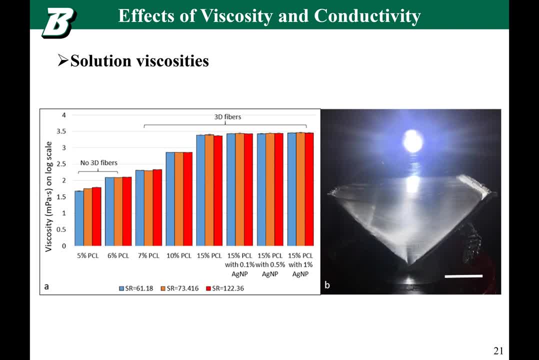 So, as you can see, we have 5%, 6%, 7%, 10% and 15% PCL solutions And we found out that when the solution viscosity or concentration is lower than the 7%, we cannot get fibers between the two bevels in 3D space. 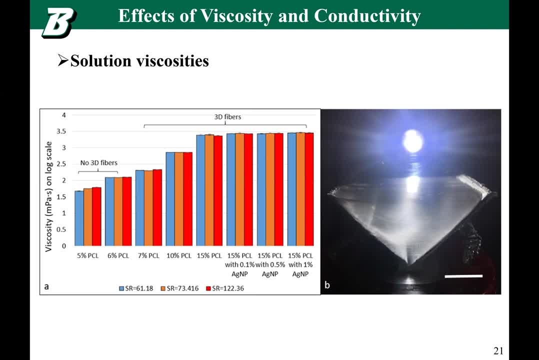 So what we're going to do is we're going to increase the solution conductivity. We're going to increase the solution conductivity. We're going to increase the solution conductivity. We can only get fibers onto the two bevels, So this means there's a threshold viscosity level for our solution to form a fibers in. 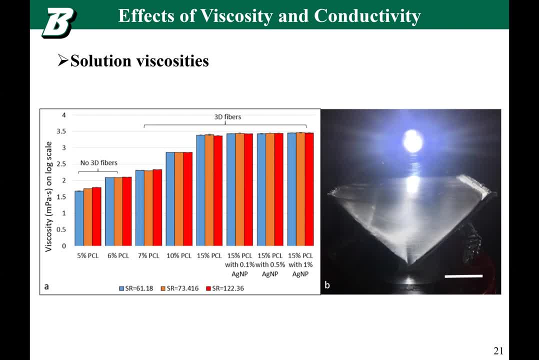 3D scale and bridge between these two bevels, And we also measured the viscosity level in different shear rates. We have three different levels of shear rate: 61%, 73% and 122%. For these three different shear rates, we did not observe significant difference between 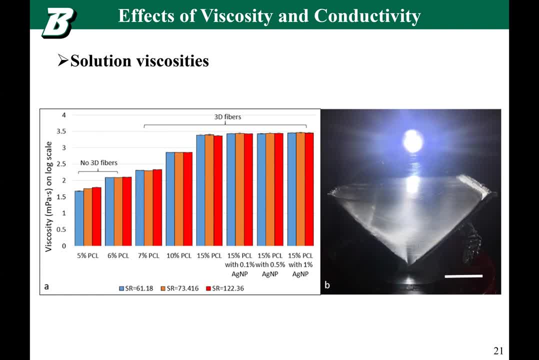 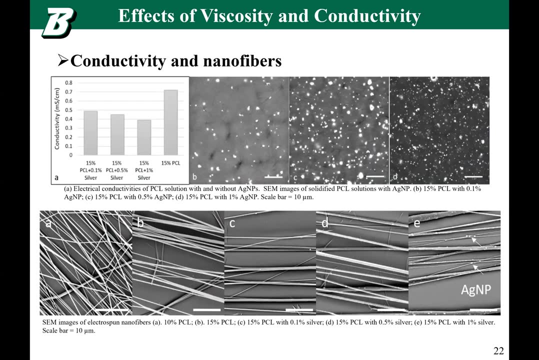 the viscosity values. This means our solution is a non-Newtonian fluid And the viscosity level will be consistent, no matter what's the shear rate. And after we have all of these scaffolds and the solutions, we characterize the conductivity of the solution. 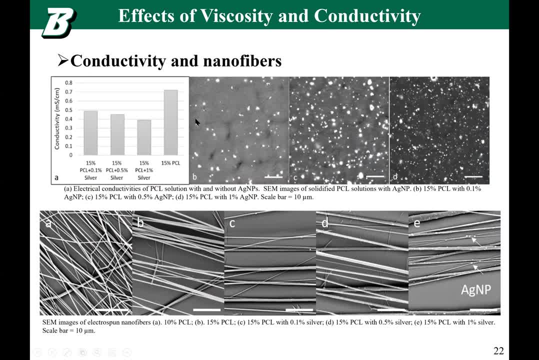 As you can see, when we incorporate the silver nanoparticles into the solution, we can observe the silver nanoparticles. However, surprisingly for the silver nanoparticles, it did not increase the conductivity, but actually decreased the conductivity of the solution. So our assumption is that the silver nanoparticle reacted with the trace element in our polymer. 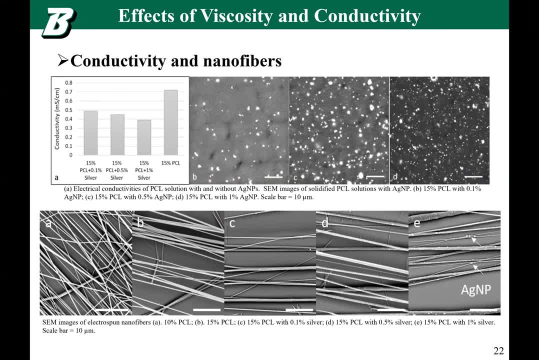 solution And the trace element in our polymer solution And all of those conductivity values below one microns per centimeter cannot be accounted as conductive for usual applications. So we also did electrospinning to fabricate the scaffold And we can see there are some silver nanoparticles on our fibers. 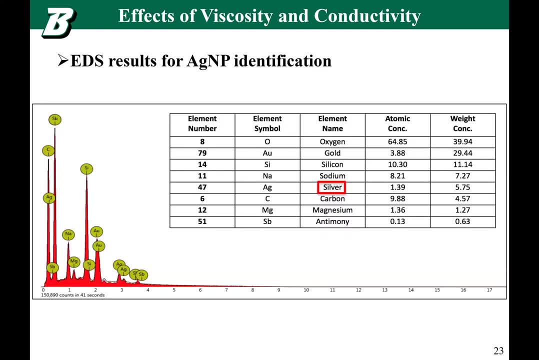 And then we did a heat transfer And we did a heat transfer, And then we did a heat transfer And we test it, And then we did a heat transfer. So we calculated heat transfer in our求se получ, However, in fact before we integrated- 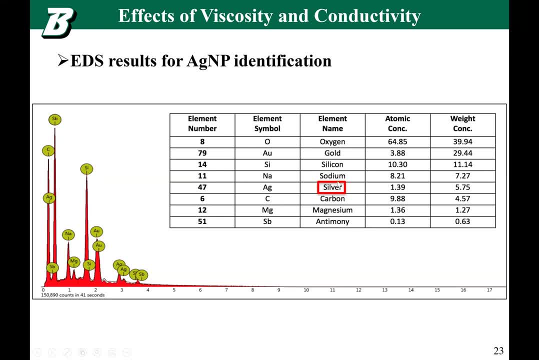 've used so called extraspinning Hard. So at this point you know we actually haven't 만 chigned then hoffe or muon, according to our huning best to a lower value to detect that there's not many. It's not like a obsession. 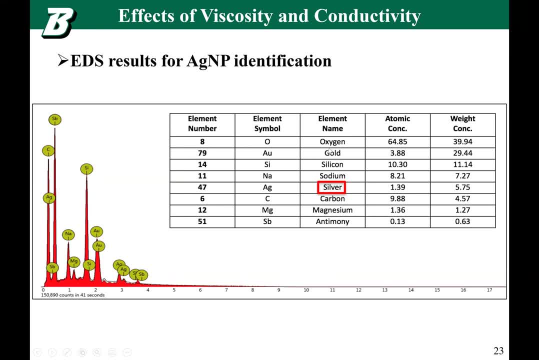 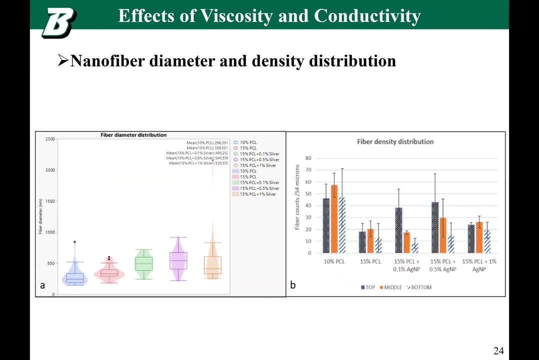 So, then, this is the. this is the result of a solid gate on the fiber, Because our heat transfer level does not increase. It is a discovered condition. It's not flat fiber diameter and fiber density analytes. we can see that when we increase the fiber. 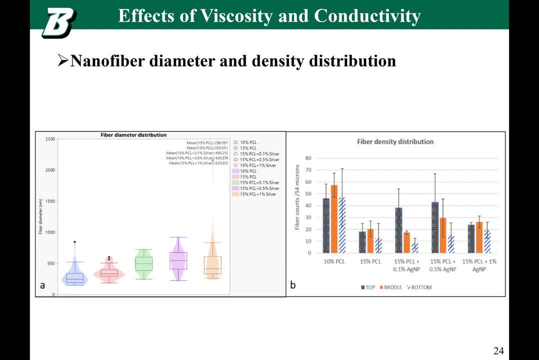 dissolution viscosity or increase the silver nanoparticle concentration, we can always get bigger fibers, But if we increase the silver nanoparticles from 0.5% to 1%, the fiber diameter actually decreased a little bit and the result in some bounding fibers that are larger than. 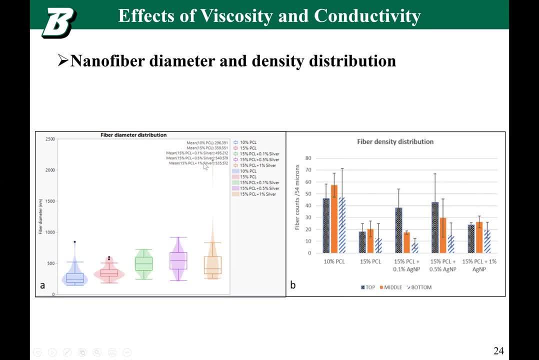 two microns, So this is not an ideal result. This means the silver nanoparticle concentration cannot be higher than 1%. in order to avoid the bounding effect for the fibers to form a micron-sized fibers And for the fiber density, we separate the scaffold. 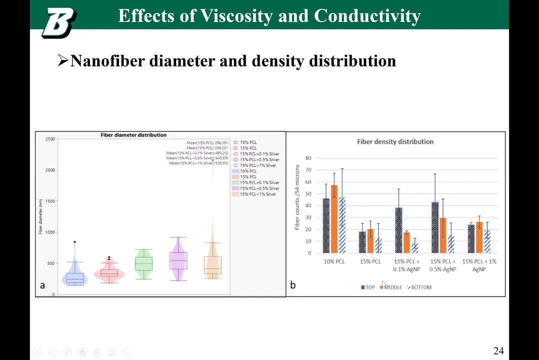 into two parts. The first part is the silver nanoparticle concentration and the second part is the silver nanoparticle concentration. And the second part is the silver nanoparticle concentration And for the top, middle and bottom sections. difference we can see when we increase the. 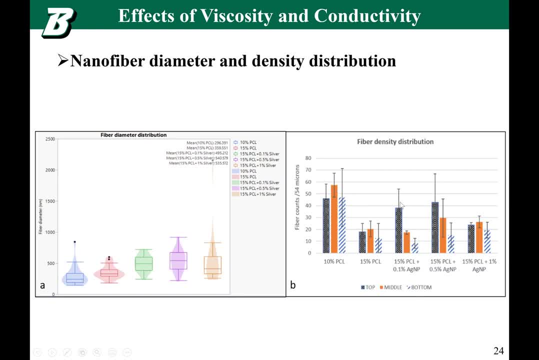 solution viscosity, we'll get higher fiber gradient, which means the difference between top section to bottom section actually increased. However, when we increase the silver nanoparticle concentration, you can see that the difference between top section all the way to bottom section actually decreased. 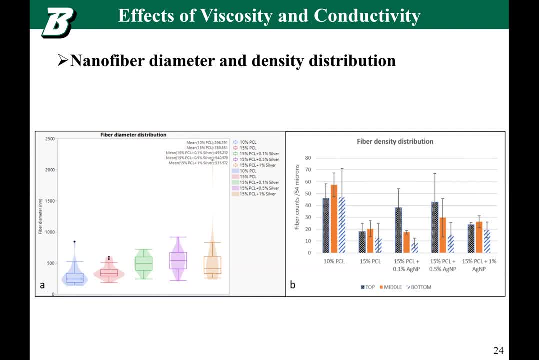 This means, if we want to increase the homogeneity of the fabricated nanofiber scaffold, we can decrease the solution viscosity or we can increase the silver nanoparticle concentration. And if you want to get a scaffold with more gradually changed features from bottom to top, you can either increase the solution concentration or decrease the silver nanoparticle concentration. 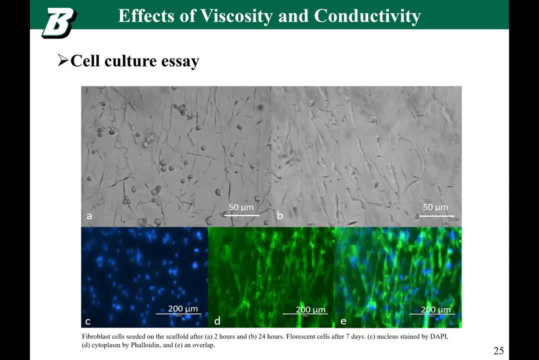 And finally, we did a cell culture to validate our scaffold or silver nanoparticle is not harmful to the cells. So the cells cultured here are human fibroblasts and after seven days we can see that the cells are already growing along the fiber structure orientation: 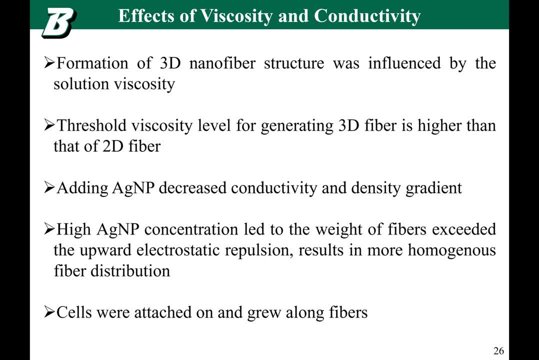 And for the solution viscosity and conductivity measure, we can see that here is the formation for 3D nanofiber structures that was influenced by the solution viscosity And there's a threshold viscosity level for GF And that threshold is higher than generating fibers in 2D space. 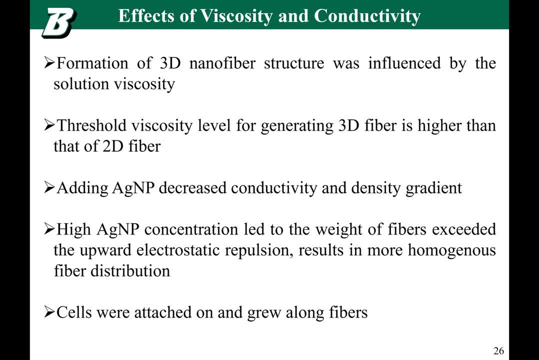 And adding silver nanoparticle actually decreased conductivity and density gradient surprisingly, And higher silver nanoparticle concentration led to the weight of fiber exceeded the upward electrostatic repulsion result in more homogeneous fiber distribution Because if we did not add the silver nanoparticle, we would not be able to generate 3D fibers. 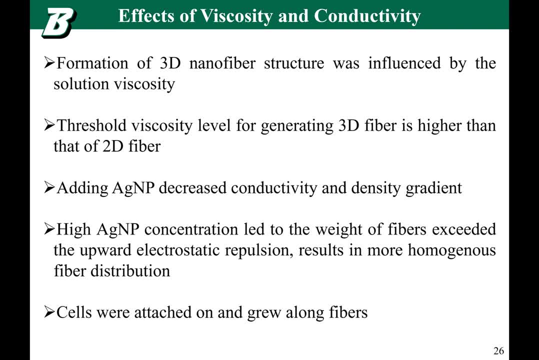 And if we did not add the silver nanoparticle, then the fibers will have electrostatic repulsion force that will repulse the fibers from depositing to the bottom and central area And cells were attached and growed along the fibers even with the silver nanoparticle incorporated. 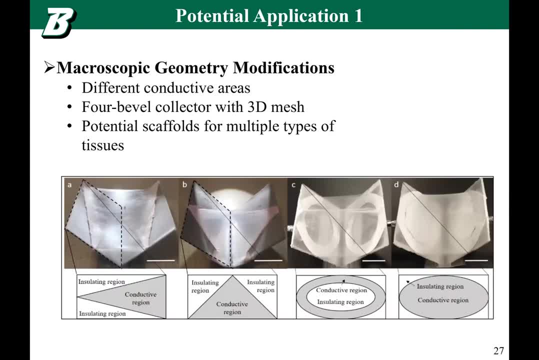 So, finally, we have some potential applications for this project. First, we can modify the conductive area on the two bevels to fabricate different macroscopic shape of scaffold, And we also fabricate a four bevel scaffold to obtain some mesh structures in 3D scale. 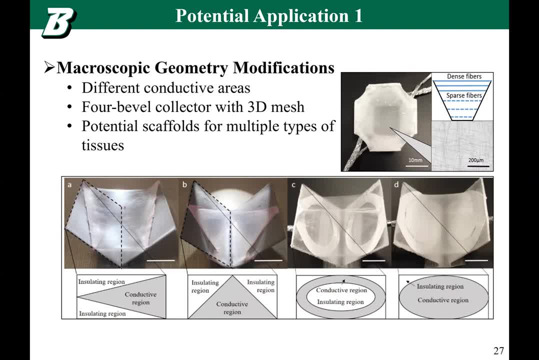 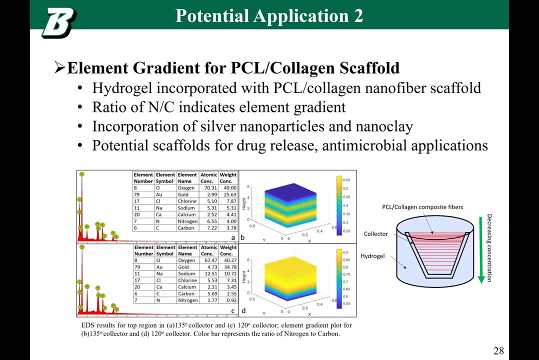 And this can be potential scaffold for multiple types of tissues. And we also incorporate hydrogel as well as collagen into our polymer solution And after we electrophene the PCL and collagen composite fibers, we incorporate this whole scaffold into hydrogel And after freeze, drying and separate the hydrogel from bottom to top sections, we can characterize if there is the collagen gradient from bottom to top. 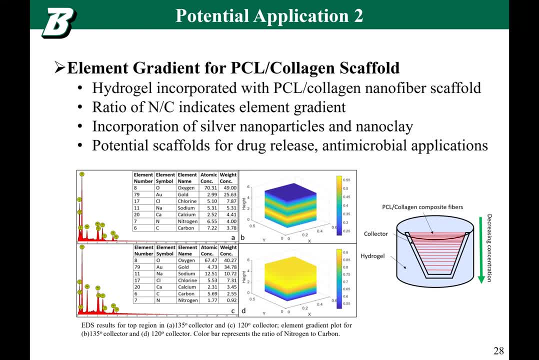 And according to our EDS results, we see that there is a great gradual change from bottom to top, or even for different tractors with different angles, there will be different gradient patterns. This can be a potential scaffold for sustainable drug release if we incorporate different drugs into our solution. 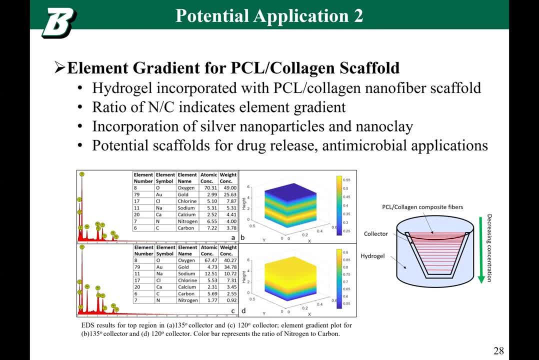 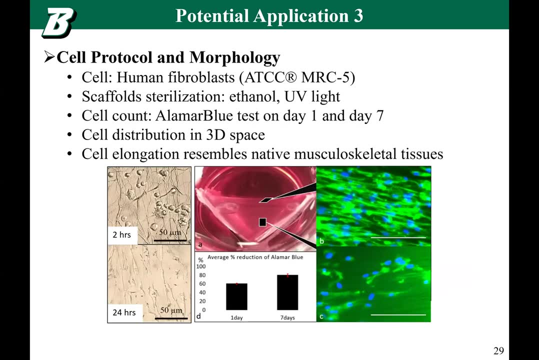 Or if we incorporate silver nanoparticles and other antimicrobial agents into our solution, we can also apply these scaffolds into antimicrobial applications. And finally, we did a cell culture for our scaffold to put the whole scaffold into a customized cell culture beaker. 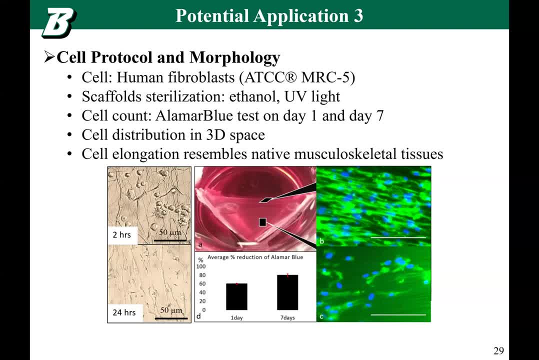 And if we put the scaffold vertically into the beaker, we can measure if there are cells on top of the scaffold as well as in front. So after 24 hours the cells had already stretched along the fiber orientation, And after seven days we can observe the cell elongation both on the top of the scaffold as well as on the front of the scaffold. 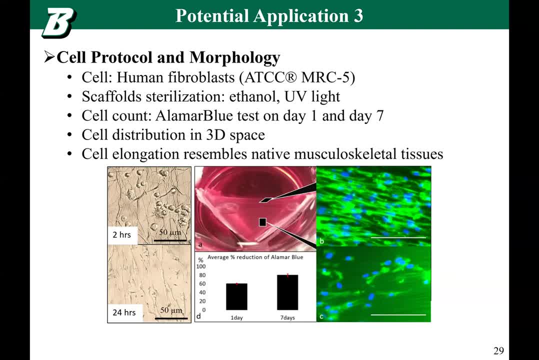 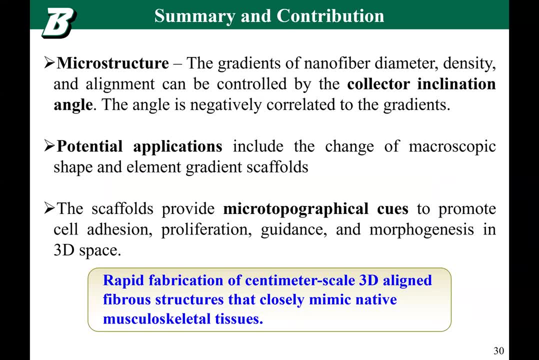 So this means the cell has been grossed in 3D space in the scaffold And the summary and the contribution is that the gradient of the scaffold has been increased Because nanofiber diameter, density and alignment can be controlled by the collector inclination angle. 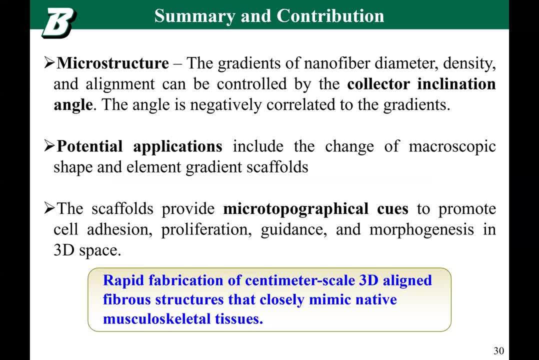 And the angle is negatively correlated to the gradient And partition applications, including the change of macroscopic shape and element gradient scaffolds. The scaffold provided micro topographical cues to promote cell adhesion, proliferation, guidance and morphogenesis in 3D space. 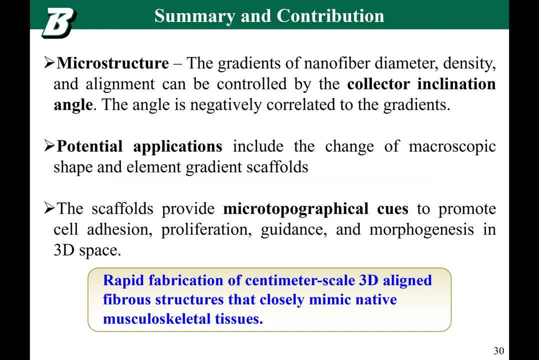 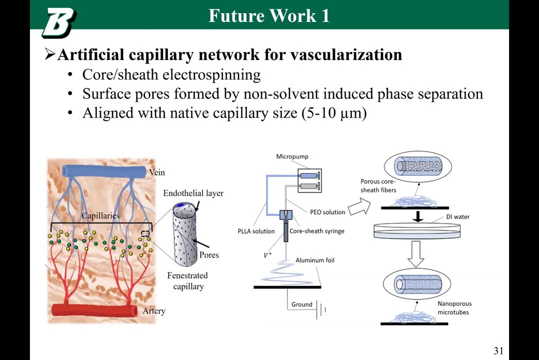 So the conclusion is that we rapidly fabricate centimeter-scale 3D-aligned nanofiber structures that closely mimic native musculoskeletal tissues. And for the future work? the first future work is to fabricate artificial capillary networks for vascularization using core sheets- electrospinning. 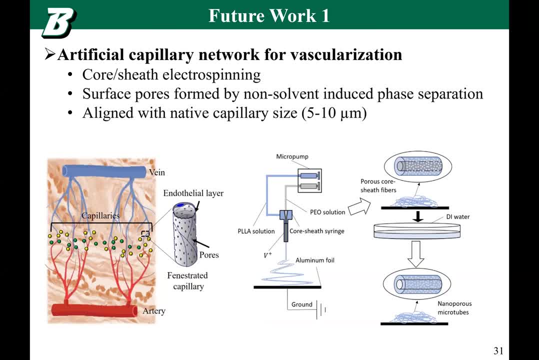 So if we incorporate a core sheet, electrospinning the core sheets spinner it into electrospinning system And we can dissolve the core in DI water. So the core will be water-dissolvable or soluble And the sheets will not be water-soluble. 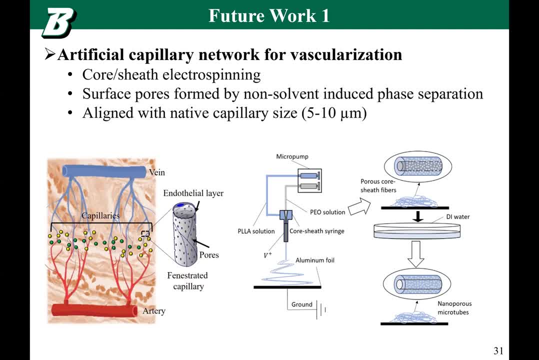 And after we dissolve it, we'll be able to obtain a nanoporous microtubular structure that is highly resembled to our human capillary structure. You can also obtain surface pores by non-solvent induced phase separation. This means if we incorporate water vapor during electrospinning process. 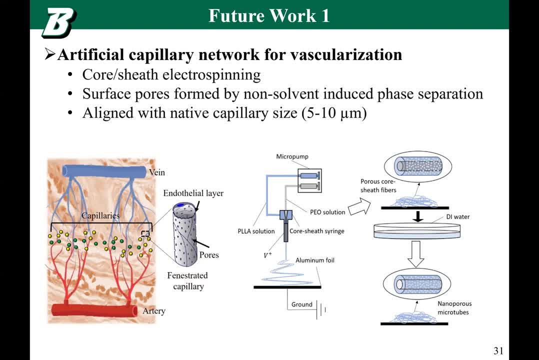 or if we're using highly volatile solvent during electrospinning process, then there will be water vapor occupying the surface of the nanofibers microtubes And then the surface will leave some porous structures. That is again highly resembled to human capillary vessels. 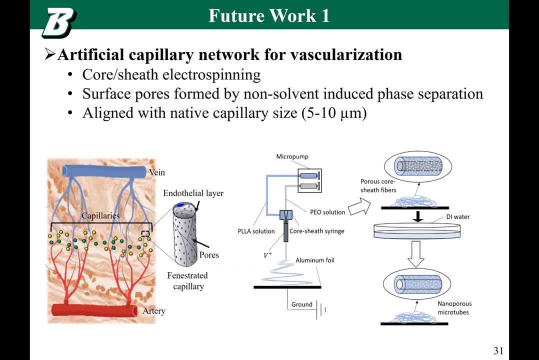 So this is an ongoing project, that several preliminary studies and pilot studies have been done, But we still need to further optimize the process and culture cells to see if it is really beneficial to cell culture, And the next future work will be hybrid biofabrication platform. 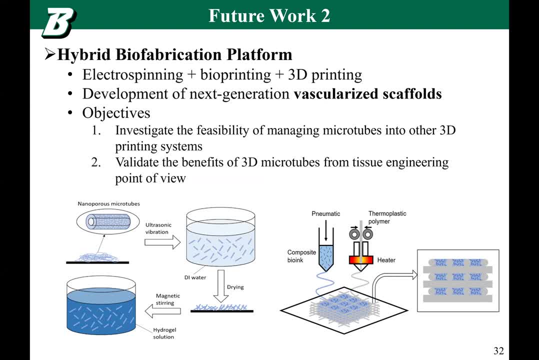 In this platform we'll incorporate electrospinning into bioprinting and 3D printing system. So after we have the nanoporous microtubular structures, we'll incorporate it into the bioink, which is the hydra for bioprinting. 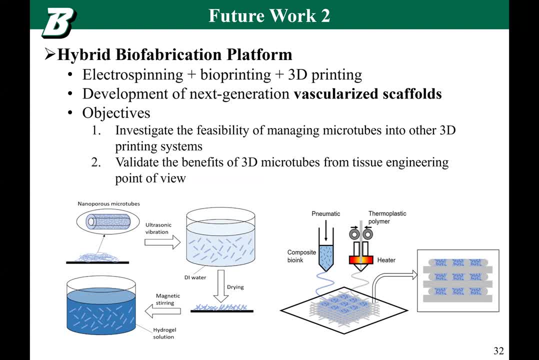 And we can print the bioprinted hydra into the gaps between FDM filaments. So in this case we'll both have the high mechanical strength and high printing fidelity for FDM, as well as the biocompatibility advantage for bioprinting. 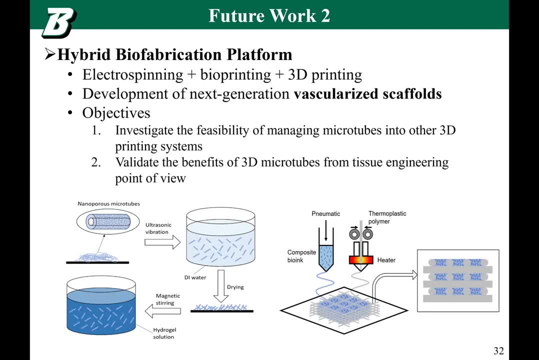 And we also have micro nanoporous structures, or microtube structures that can function as capillary blood vessels for cells inside of the hydrogel. So in this case we can investigate the feasibility of managing microtubes into other 3D printing systems. 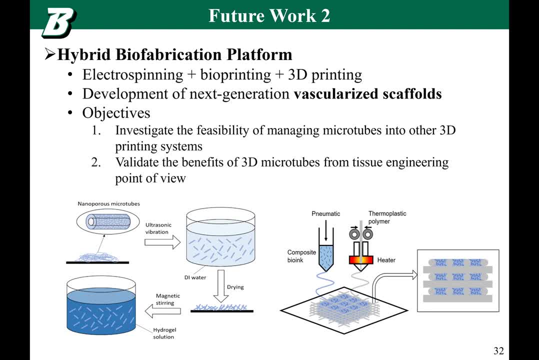 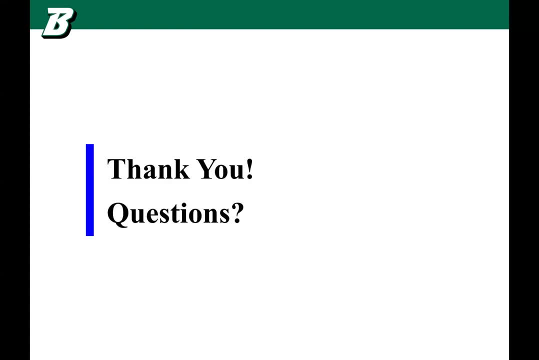 and also to validate the benefits of 3D microtubes from tissue engineering point of view. So this will be concluded, all of today's presentation. Thank you very much for this opportunity and I'll be happy to take any questions and comments. 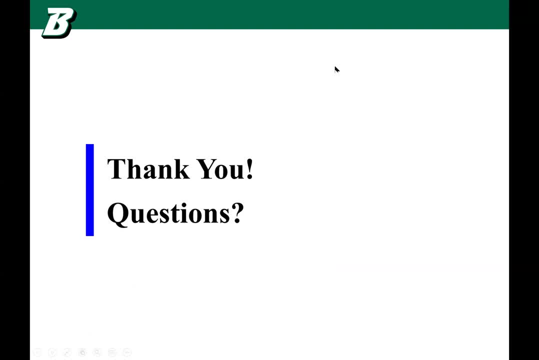 Joe, thank you very much for your presentation. It's definitely nice to hear about your work and to learn about some of the tissue engineering activities that are taking place in your lab. Thank you. At this point, I'd like to open it up for questions. 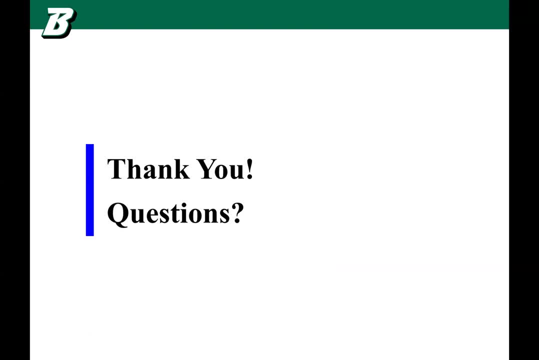 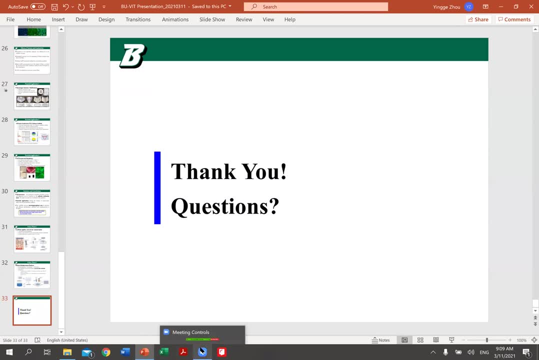 Again, please feel free to unmute yourself and ask the questions. Yes, Prabhu, Yes, please, Yes, thank you for letting me ask the first question, Professor Zhao. this is very interesting, very nice talk. I want to know whether this technique of electrospinning and related techniques can be used to develop skin tissues. So, for example, a patient who has burn injuries, can this technique be used to develop artificial skin? Besides biomimetic scaffolds for tissues within the body? Sure, I think electrospinning has very extensive applications on the wood dressing. So, for example, if we have a burned tissue, we can spray electrospinning fibers onto the skin directly and to form a protective mat. 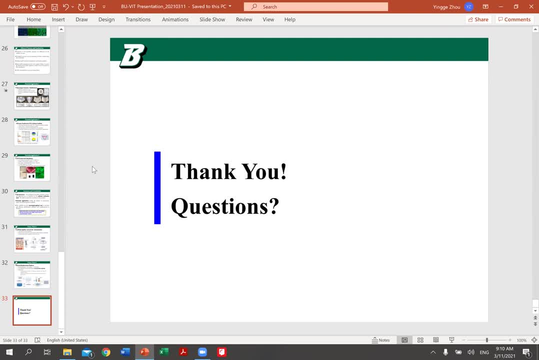 And because of that it's very effective And because it's a nanofibers mat, it can be very beneficial for the skin to heal and can be protected from the infection. If we incorporate some disinfection factors into the electrospinning solution and we spray these nanofibers onto our skin, it would be very beneficial for skin to heal. 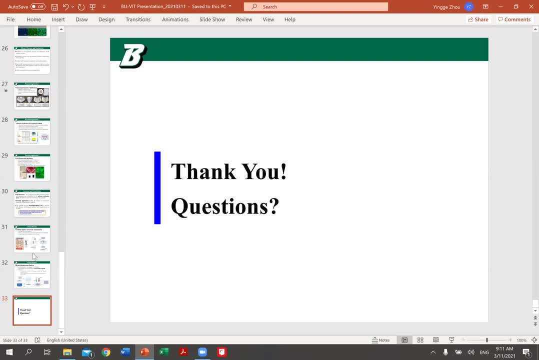 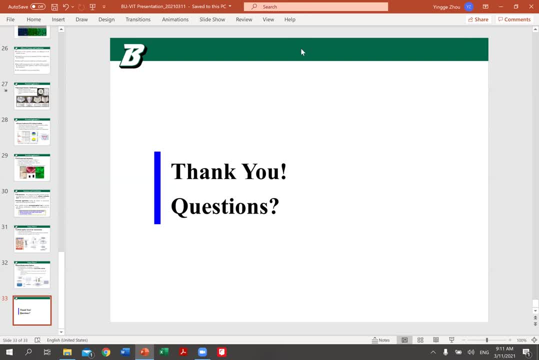 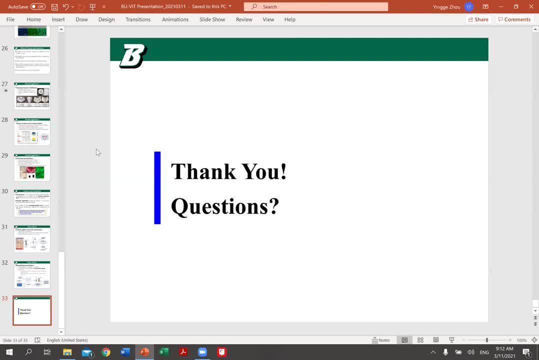 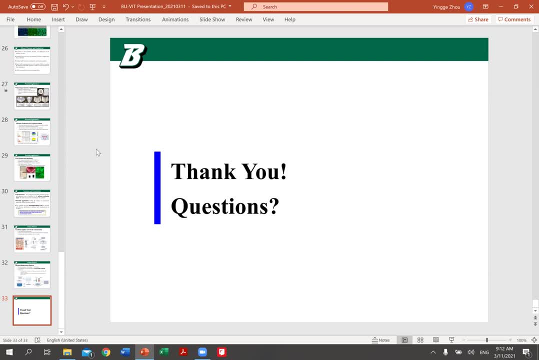 dinner a little earlier than usual, So it will be one hour earlier for us and one hour earlier for our colleagues in India. Bruno, I'm not sure. I think in your case also it will change. Yes, also in my case it will change. one hour before. 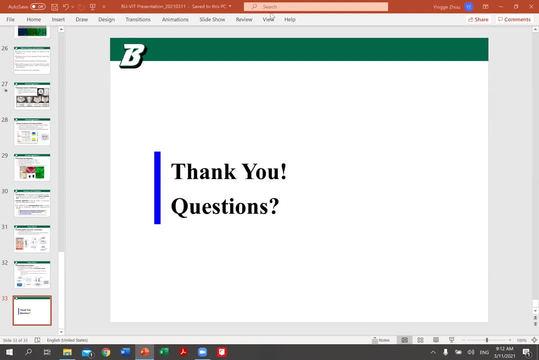 Yes, one hour In Europe. the time changes at the end of this month, The last Saturday of this month. that will be the time change. Any other questions? for Dr Joe, I could ask a second question. Oh yes, please. 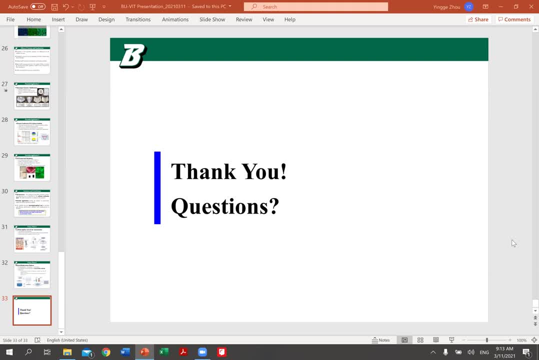 Yeah, So the thought that went through my mind was related to the reliability in the actual field. So, for example, we apply this tissue inside the body or on the surface of the skin, How long will they last? And for example, 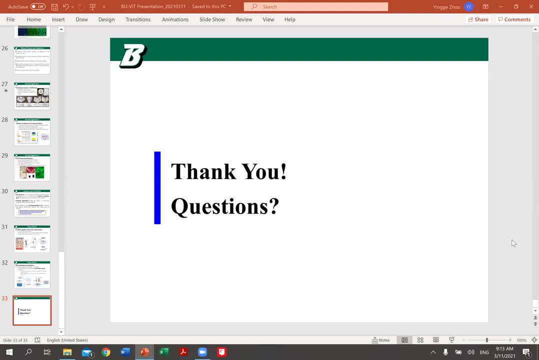 how? I mean, is it going to be years before they need a replacement? Is there any such research that has been done? Can you please throw some light on it? Sure, Although the biometric application of this electrospinning technique may be not my research focus, but I 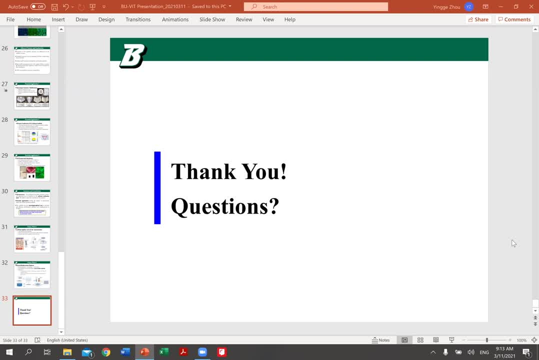 do have some reading about it, I think the first: the electrospinning fiber has to be biocompatible and it should be decomposed after several, probably I would say several- months, And it won't be harmful to humans even if it's inside of the 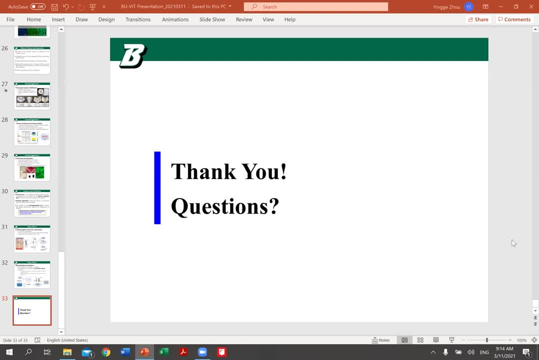 human body because we're, you know, using biocompatible and degradable materials. So, as for your question in terms of what happened after inciting the human bodies, or how long exactly it will take, that one I'm not really sure, because 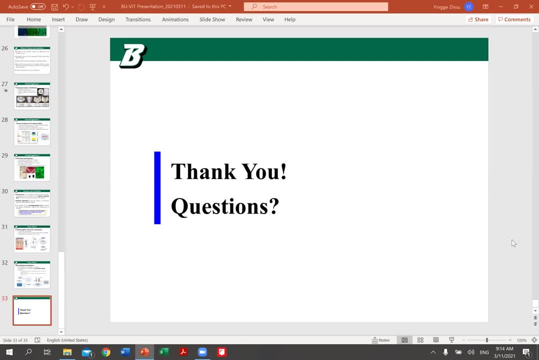 it's not, probably not my research focus. Okay, Yeah, Thank you, Thank you. Thank you, Prabhu. Thank you. Any other questions? Please don't be shy. Okay, so if there are no questions, we can end the session. 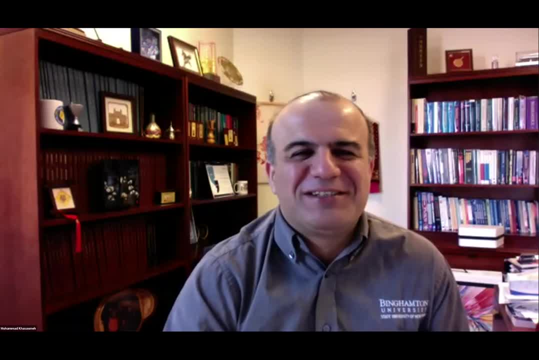 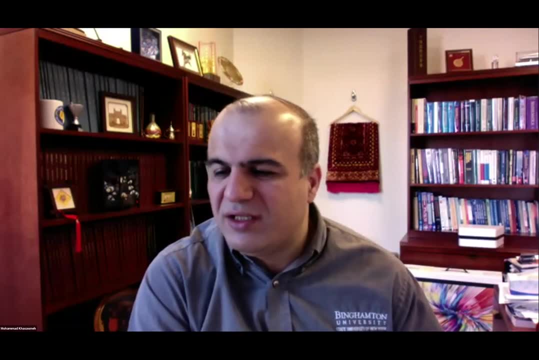 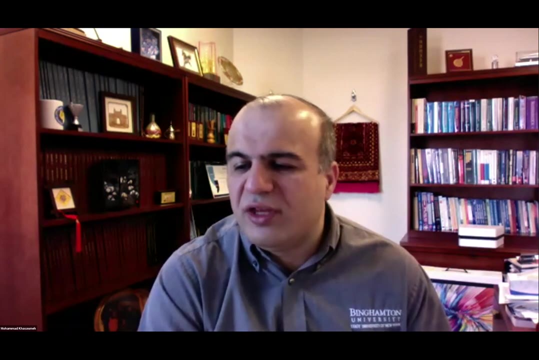 earlier this time. Usually we are a few minutes behind schedule and we end up taking a few minutes extra. Oh, there is one professor, Professor Kanna Dasan from VIT, asking if you can share your views on 3D printing of organs. 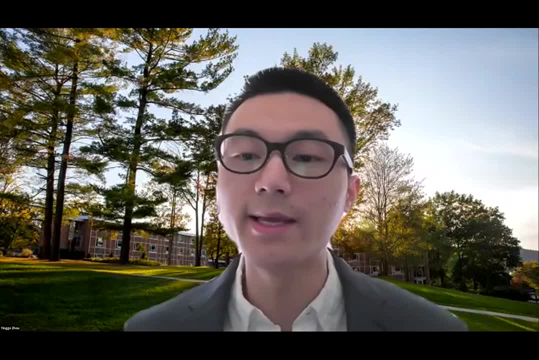 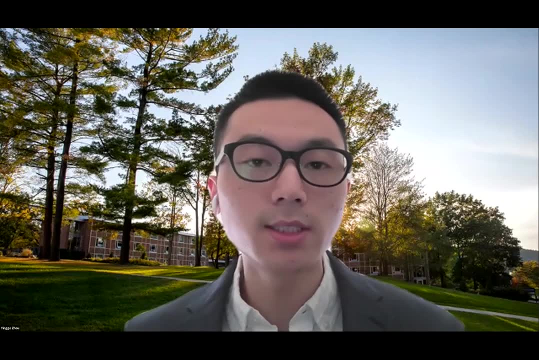 Yes, sure, 3D printing of organs is definitely a very fascinating field and an emerging research area, But I do think there's a few key challenges to be addressed before it can be scaled up or can be applied into industrial. First challenge is: we cannot print capillary vessels or even artery and veins inside of the printed tissues. It is very hard to do that while we're printing the organs, but without the blood vessels the cells cannot survive inside of the organs because the culture medians are just. 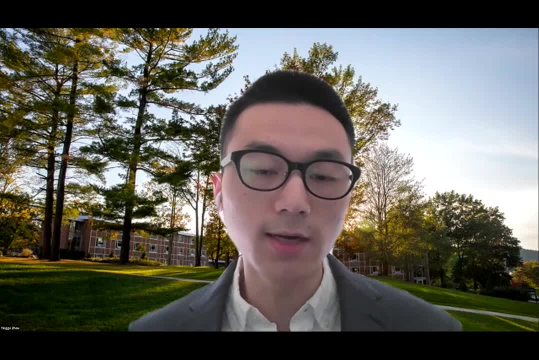 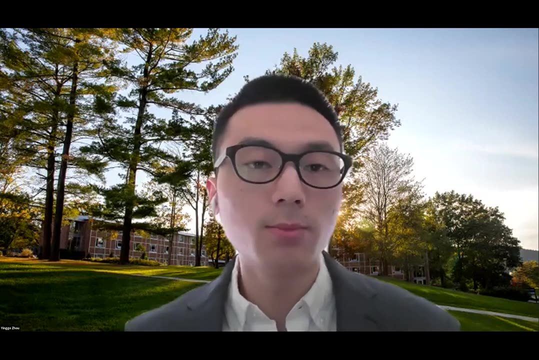 surrounding the tissue. There's no nose in the heart, there's no nose in the blood vessels, so there's no blood knows enough nutrition or transplantation of waste for the cells to live or survive. The second one is: the second challenge is that 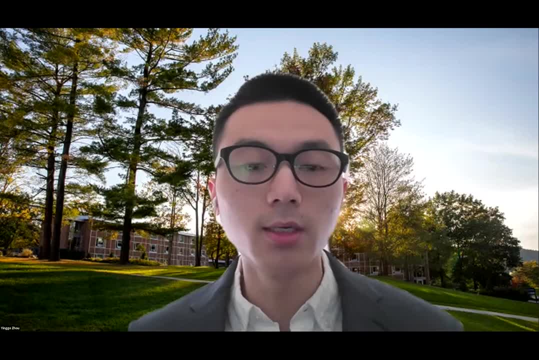 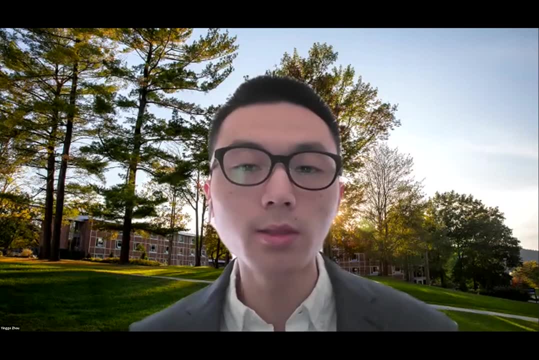 probably a lot of researchers is already addressing it. So it's the composite materials. So because one tissue has a lot of different materials and a lot of geometries, so how to print those different materials at one time and incorporate to each other using different printing technologies? 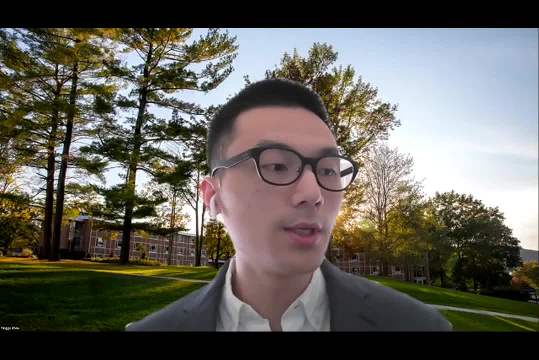 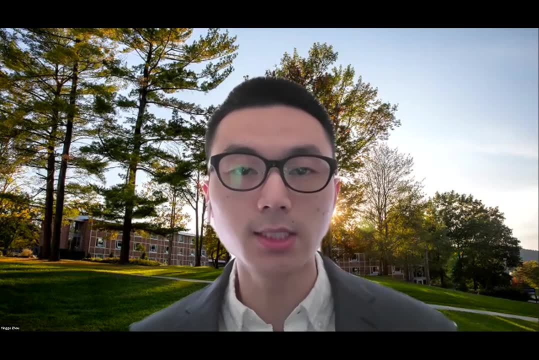 such as 3D printing, bioprinting or even STL, steel lithography and other techniques can be incorporated together to incorporate those different composite materials so that we can better mimic the native tissues. So I think those two challenges has to be addressed. 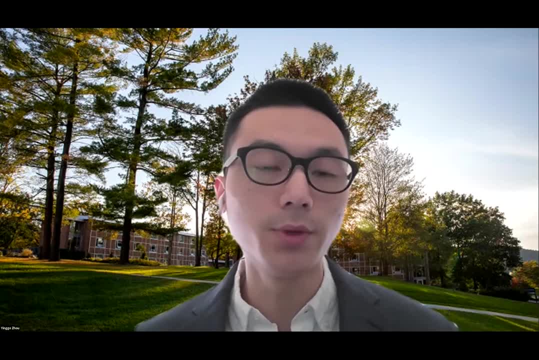 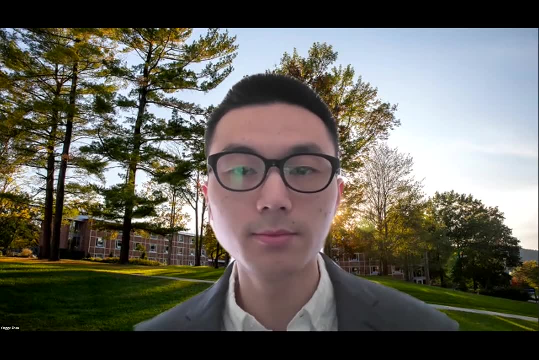 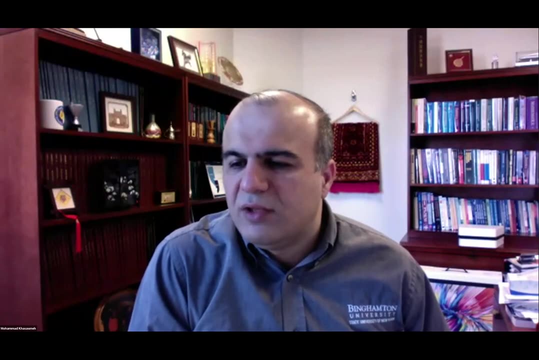 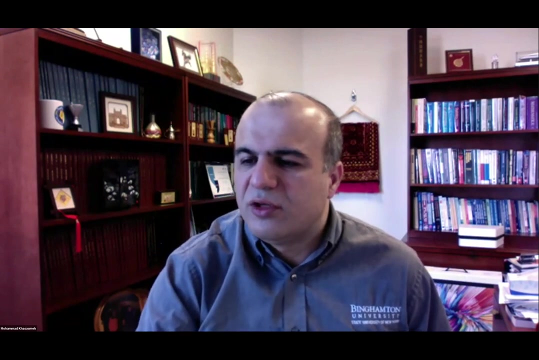 before 3D printing of organ can be really realized in like clinical scale. Okay, great, Thank you, Dr Zhou. Thank you Any other questions? Just go through the chat again to make sure I don't miss any Questions or comments. 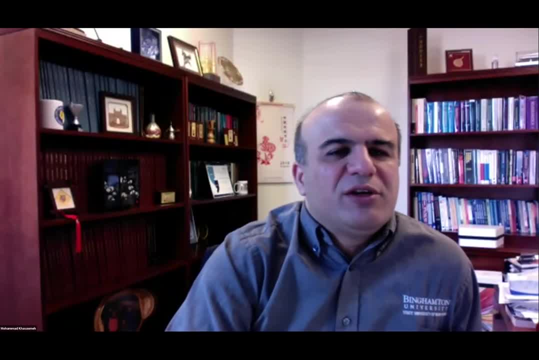 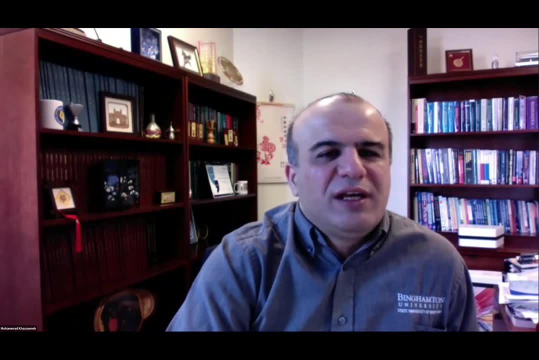 Okay, looks like there are no more questions. Dr Zhou, thank you again very much for your time. On behalf of Binghamton University and VIT, Dean Vasudevan and I would like to thank you for taking the time to join us today. 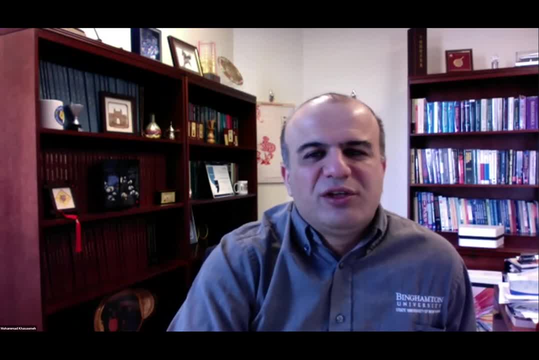 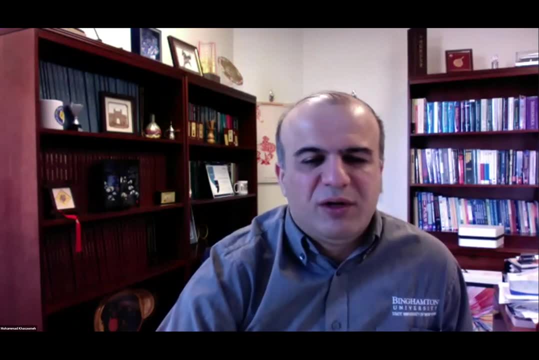 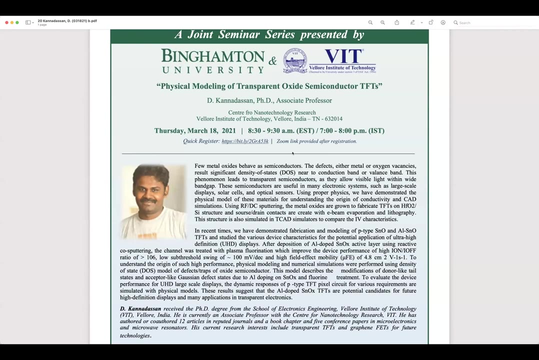 to talk about your research. We definitely appreciate your contribution. Thank you, And before we conclude, I'd like to remind everyone about next week's talk. Next week's talk will be by Dr Khanna Dasan, who's an associate professor at VIT. 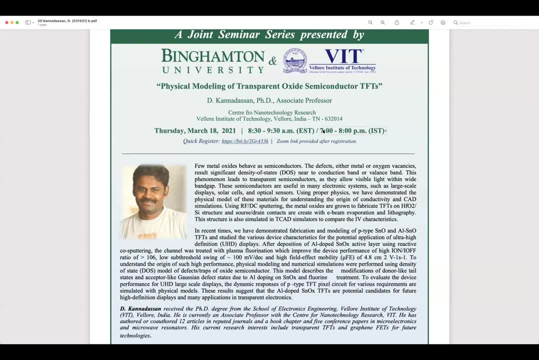 Yeah, please ignore this time. It's just 7 pm but because of the daylight saving we'll change it to 6 pm. But Dr Khanna Dasan will talk about physical modeling of transparent oxide semiconductor- TFTs. 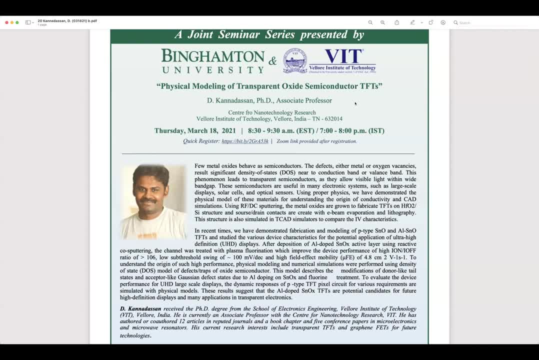 So I hope that many of you will be able to join us next week to listen to Dr Khanna Dasan's presentation And, as usual, I will be sending out a recording of Dr Zhou's presentation with a formal announcement about next week's presentation. 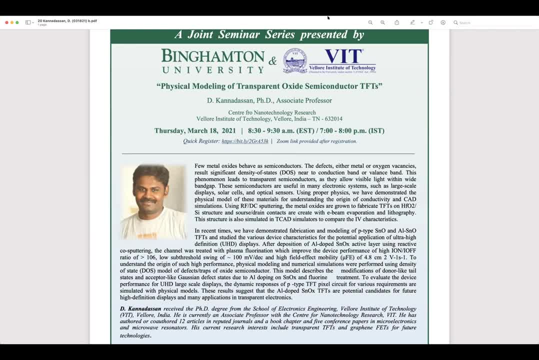 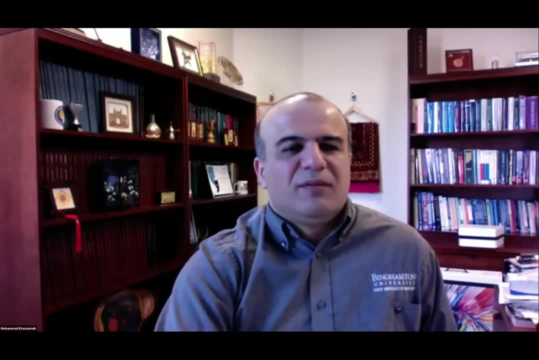 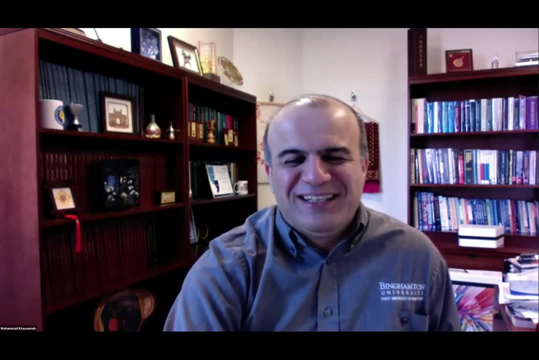 And please feel free to share this with your students, colleagues, friends, and encourage them to you know, participate. And with that, thank you very much again. everyone, Have a wonderful evening if you are in India. a great afternoon if you are in Italy. 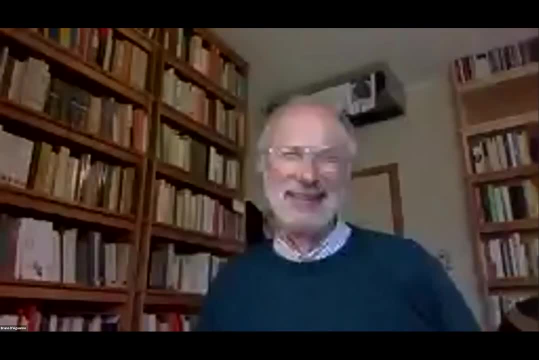